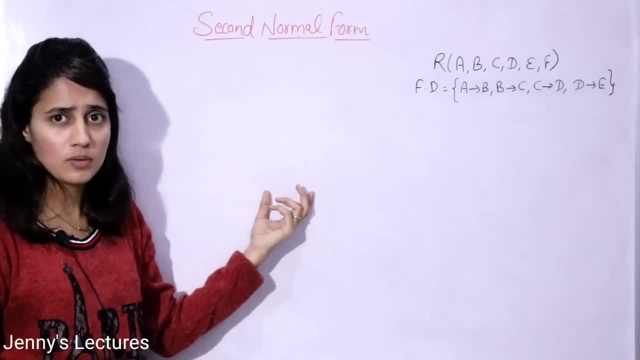 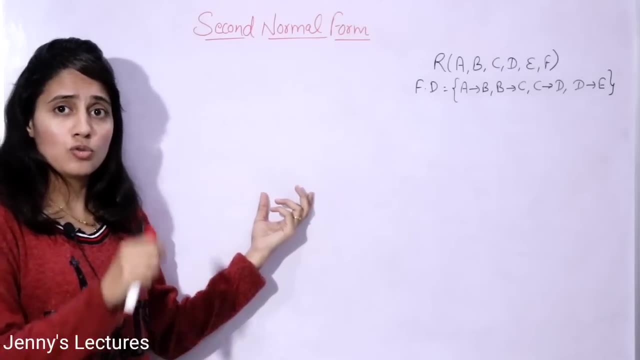 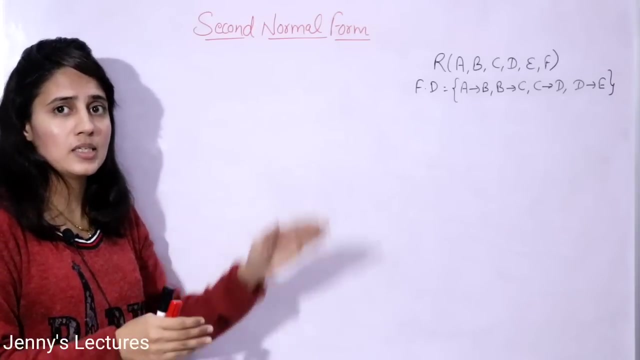 will ask that tell me this table is in first normal form or not, right? Because first normal form is the basic point, the basic step of normalization. So always they will give you a table or the schema in first normal form. Now the important point is you have to identify that as in second. 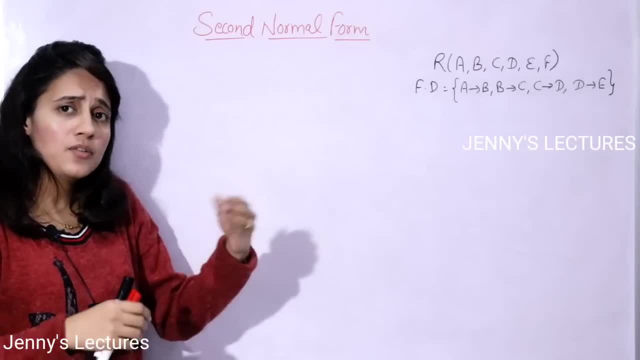 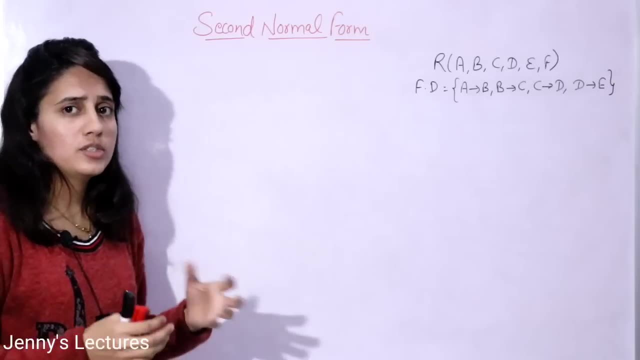 normal form. third normal form: BCNF, something like this, And if not, then convert it into the desired normal form Right. So in gate and net, these type of questions will be asked. They will give you these type of. 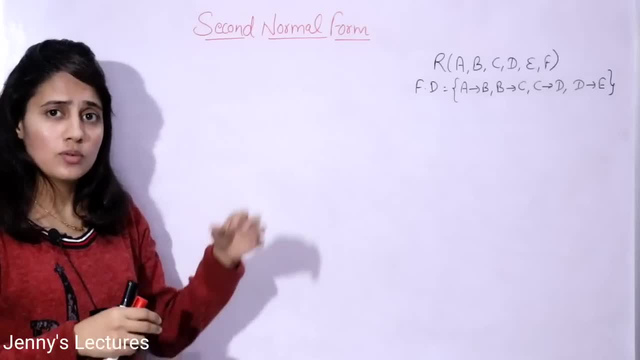 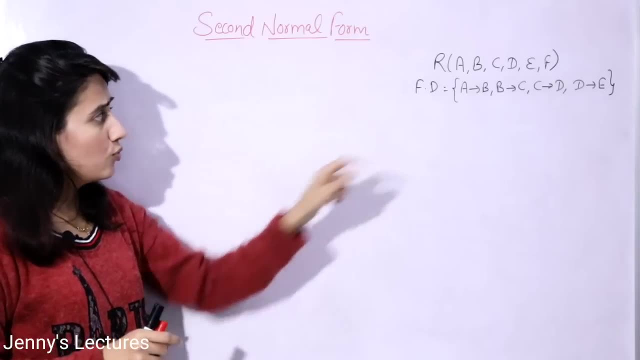 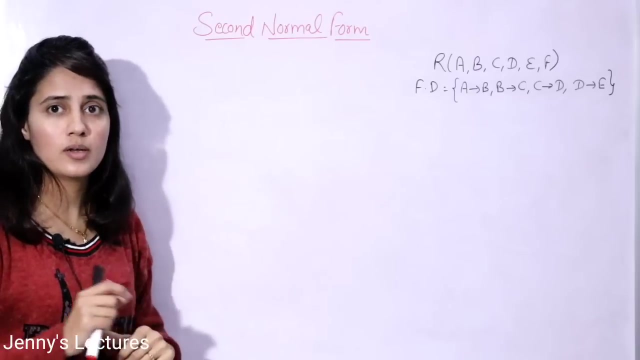 questions. Functional dependencies are given and they will ask you that: which highest normal form is there in this relation? So you have to find it out. So we have only functional dependencies, right? So this functional dependencies will play very important role here. So I have already 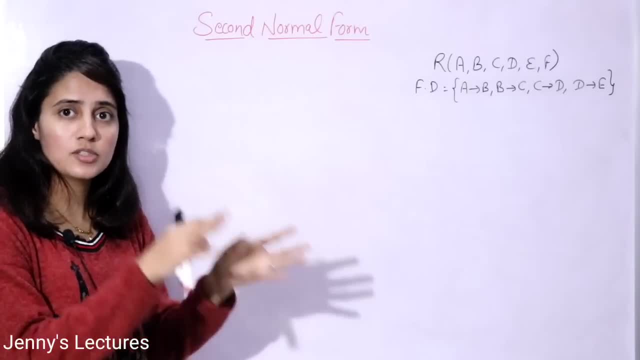 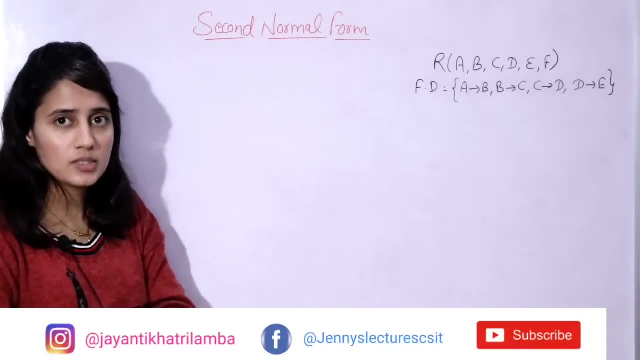 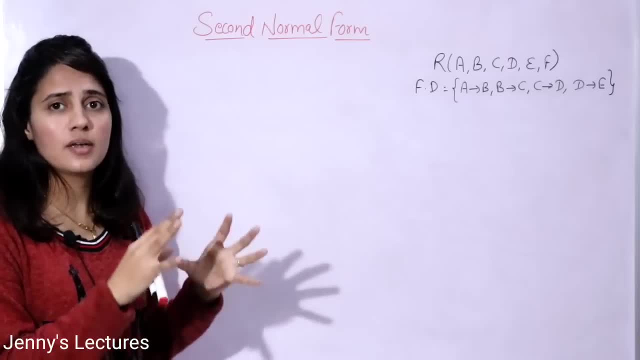 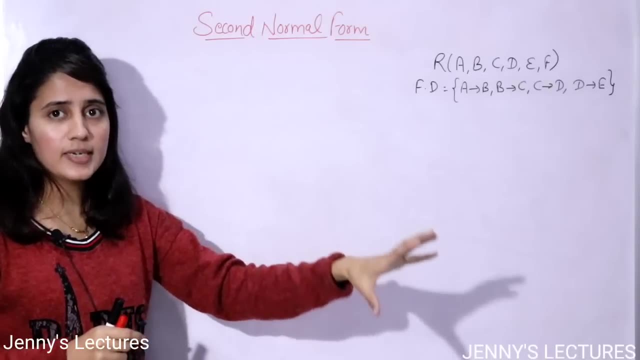 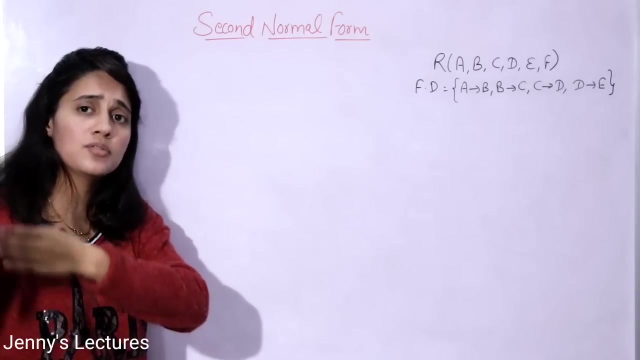 know how to calculate candidate keys. in a relation, Candidate keys plays very important role. Without finding out the candidate keys, you cannot solve the problem of normalization: Second normal form. third normal form- BCNF. fourth normal form- BCNF, and so on. So you have to find out the problem of 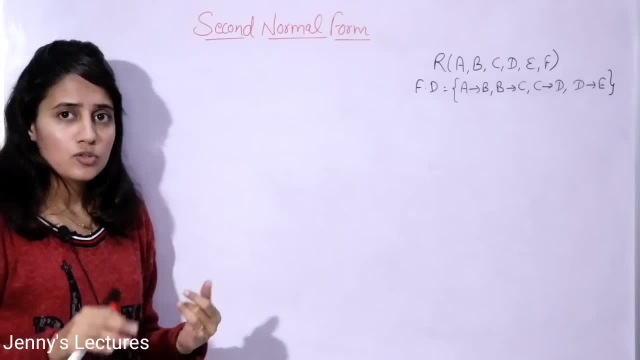 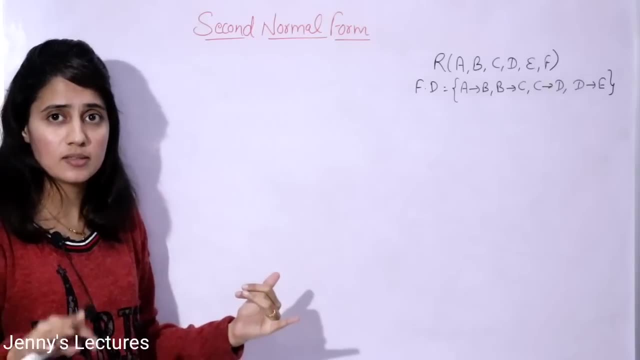 normalization: Second normal form, third normal form: BCNF, fourth normal form: BCNF, and so on. So candidates keys: you should know that also we have discussed how to find out candidates keys in a given relation. All the candidates keys, Not one. all candidates keys right, with a simple trick. So 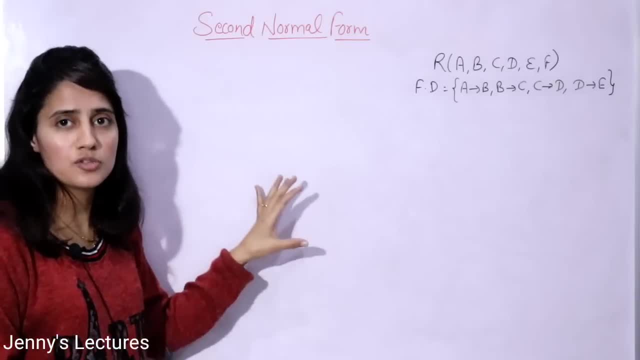 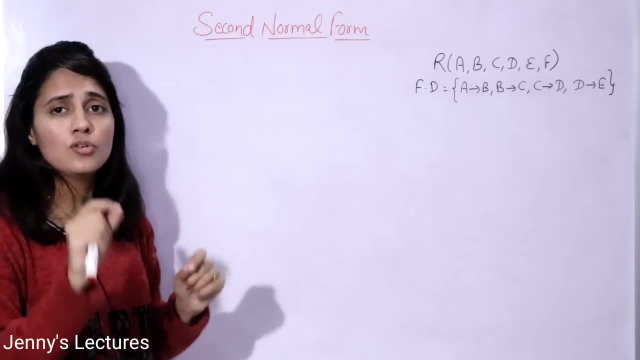 you can check out that video in the side button right And after that come to this video. So now in this video we will discuss how to find out that particular given relation is in second normal form or not right. What are the rules? 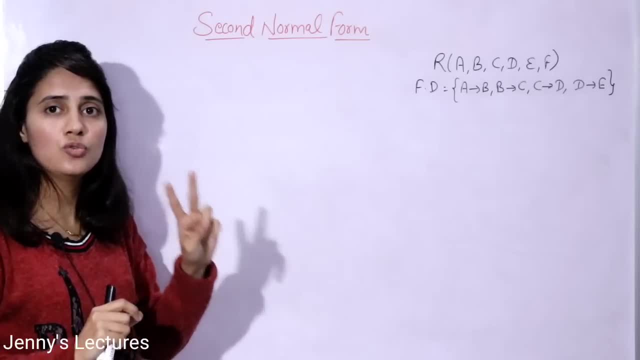 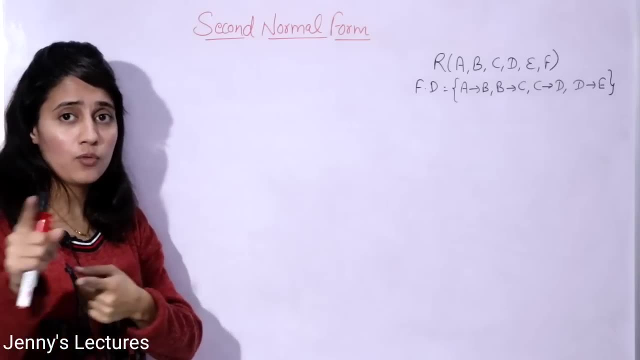 for a relation For the second normal form. what are the rules for the relationship? Can you tell for a relation to be in second normal form? there are basically two rules. first rule is very simple: that that relation should be in first normal form and i have already told you if they'll. 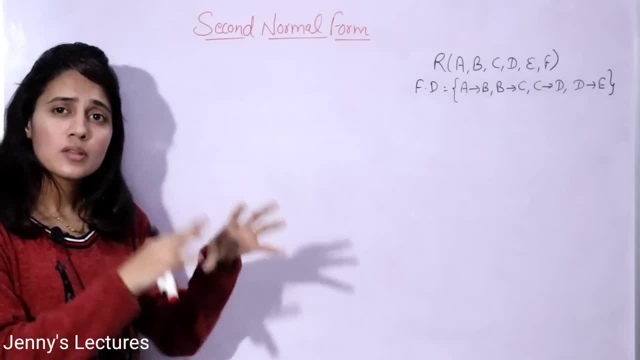 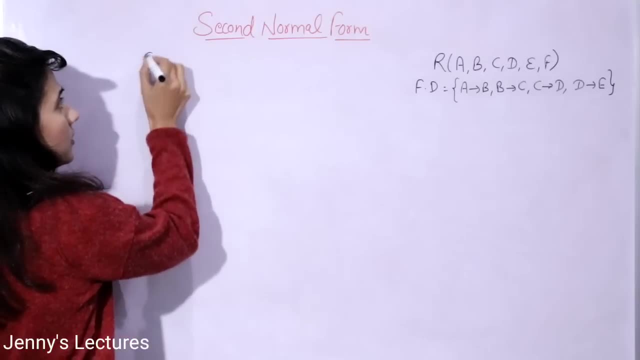 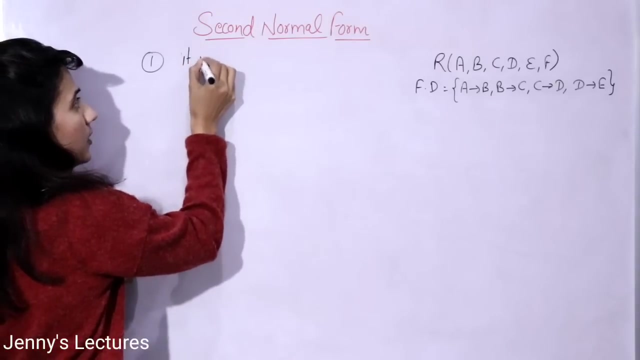 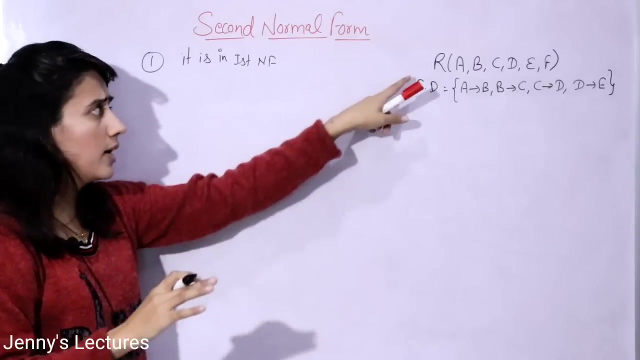 give you this type of question, that a relational schema is given that is by default that will be in first normal form, right. so first rule is a relation is said to be in second normal form. if first rule is, if it is in first normal form, right, and this already we by default, we consider that this is in first normal. 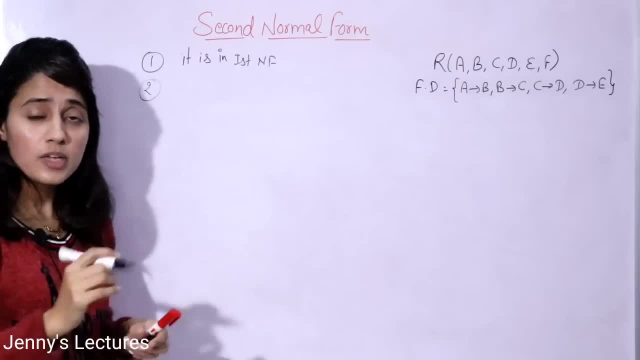 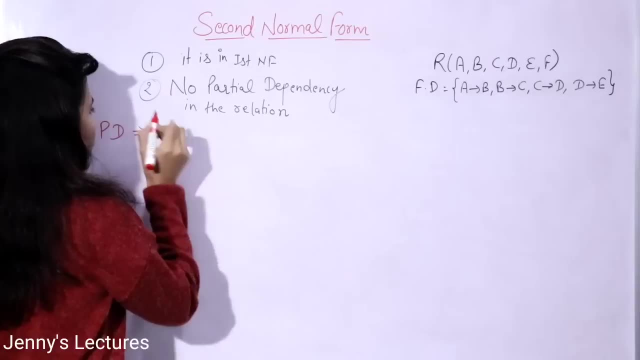 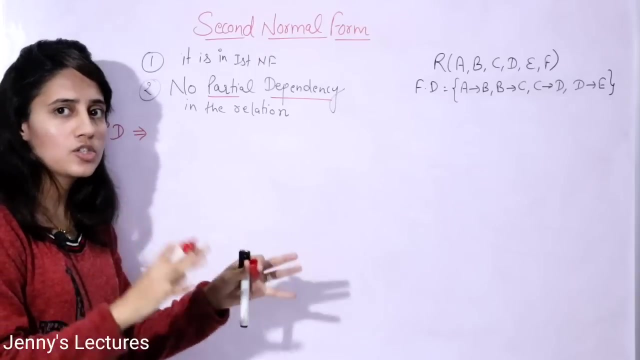 form right. second rule is what: there would be no partial dependency present in the relation. now, what is partial dependency? that also i'll discuss. so this: what is this partial dependency? now, i hope everybody knows what is functional dependency and what is partial dependency. now, i hope everybody knows what is functional. 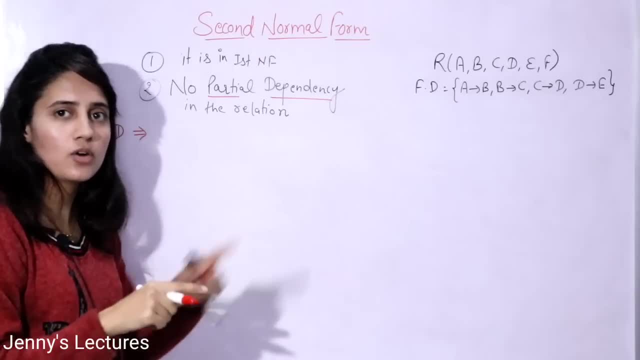 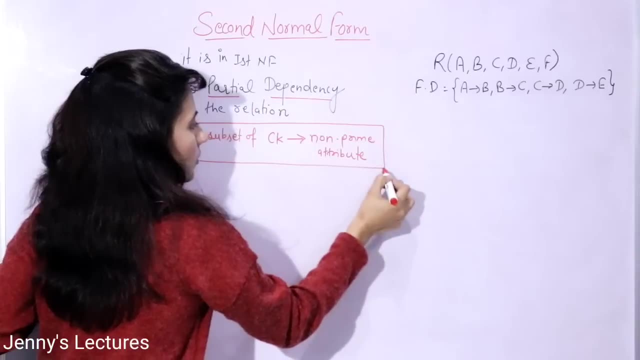 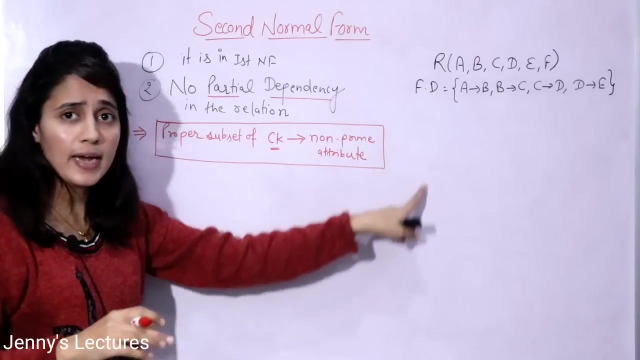 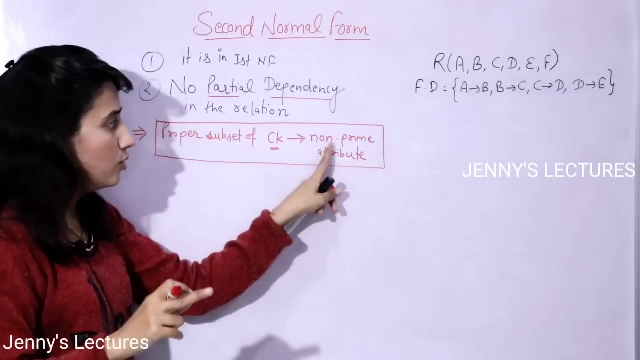 dependency. right, i have already discussed- you can check out that video in the side button now- what is partial functional dependency. or you can write down it something like this: proper subset of candidate key, of any candidate key. if suppose there are three candidate keys, so proper subset of any candidate key will determine. 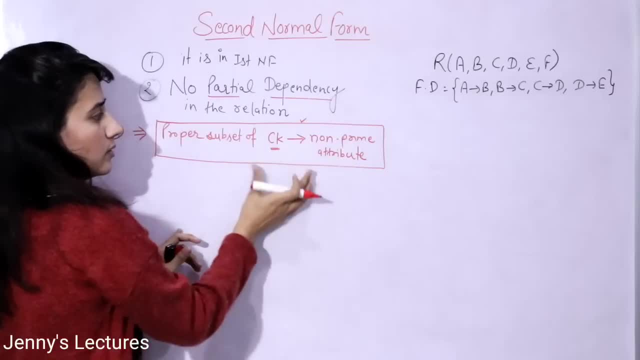 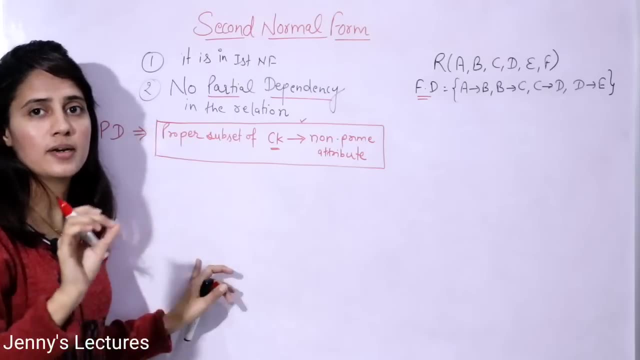 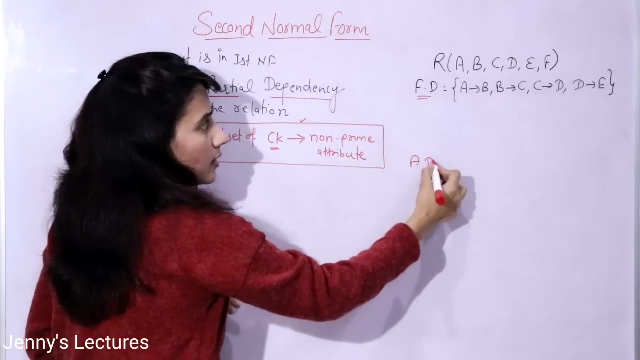 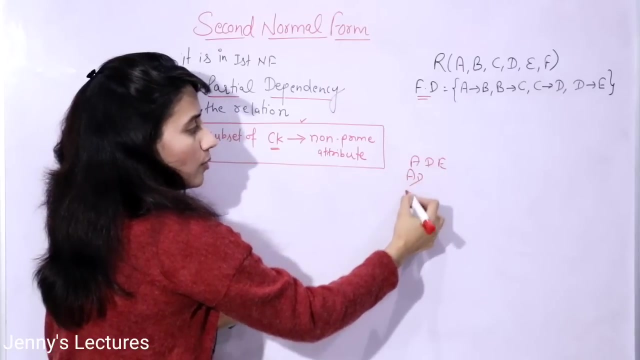 known prime attribute. if this kind of dependency is there in the list of functional dependency given, then that is known as partial dependency. right, proper subset of candidate key: see suppose candidate key here is a, d, e. so proper subset of this is what a, d is also proper subset, d e is also proper subset, or you can write a e. 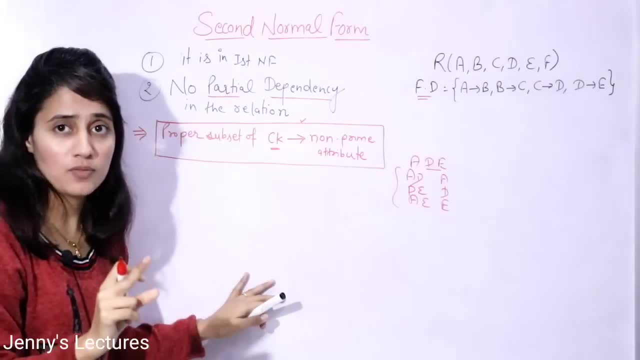 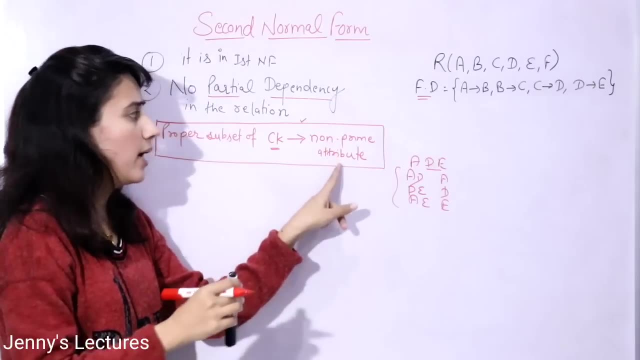 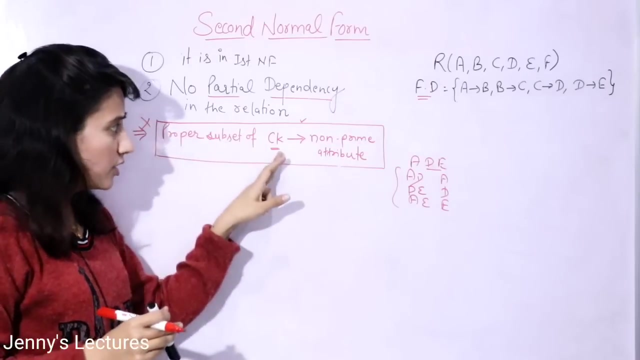 a, d, e, six proper subset of. are there right? so if any proper subset of the candidate key will determine the known prime attribute, then that is partial dependency and that should not present in the relation. if partial dependency is there in the relation, that then that relation is not in second normal form. 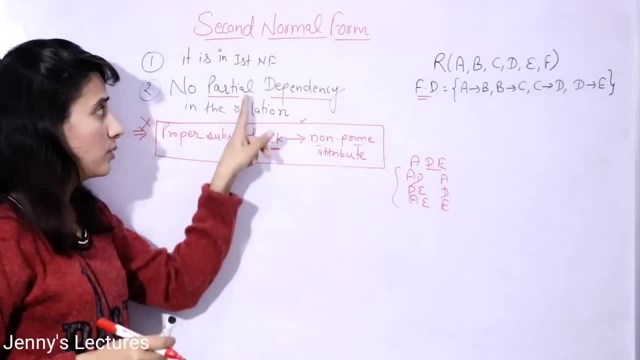 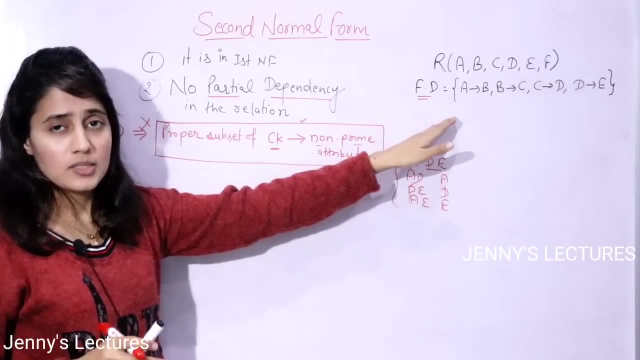 now, what is this known prime attribute? i hope you got what is partial dependency right. partial functional dependency. you can say now: obviously i'll discuss this with the help of this example, then you will get it better. now, what is known prime attribute? see, i have already discussed prime. 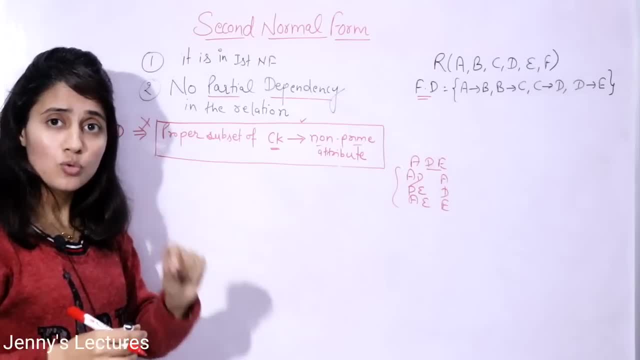 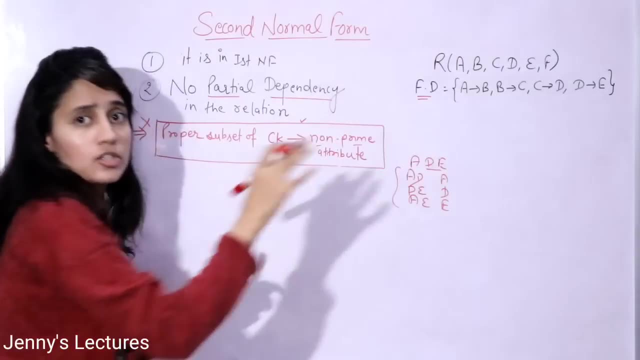 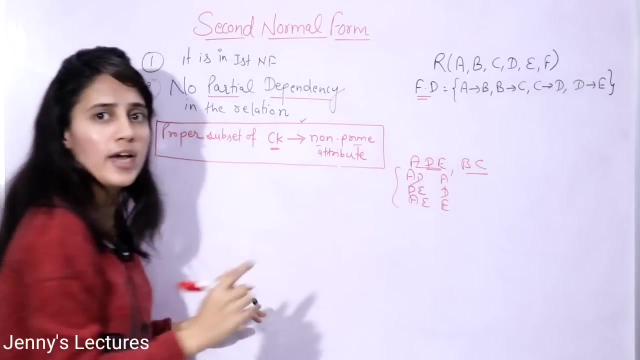 attribute, known prime attribute. prime attributes are those which are part of candidate keys, right suppose, here in this relation, suppose i'm not saying that these are the candidate keys. suppose a, d is candidate key, b c is candidate key, two candidate keys are there in this relation, right? so prime attributes would be what? 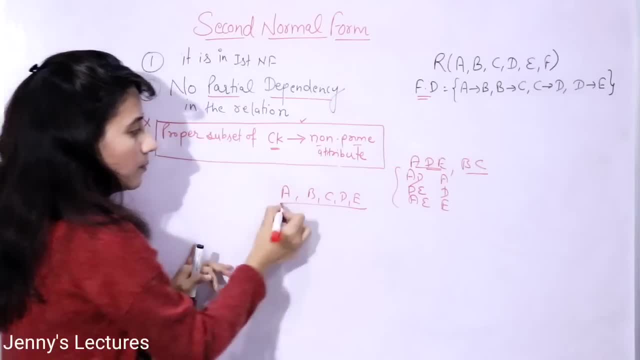 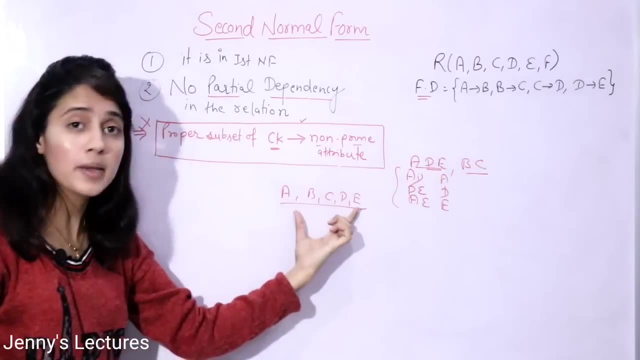 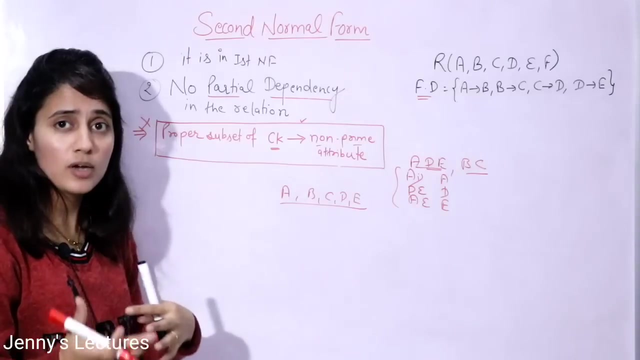 a, b, c, d, e, the attributes which are part of candidate keys or which are making the candidate key, those are prime attributes and the remaining attributes are means. the attributes which are not part of candidate key, which are, those are known prime attributes. so here known prime attribute would be: i guess only f would be known prime. 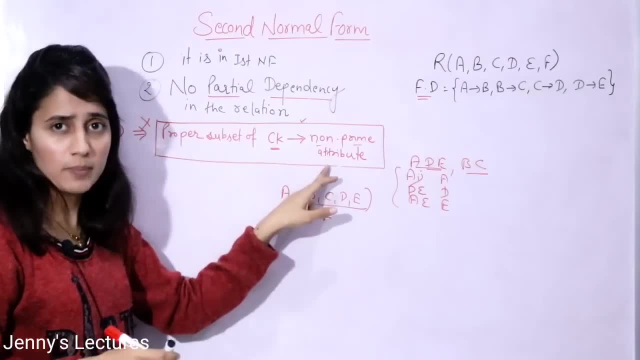 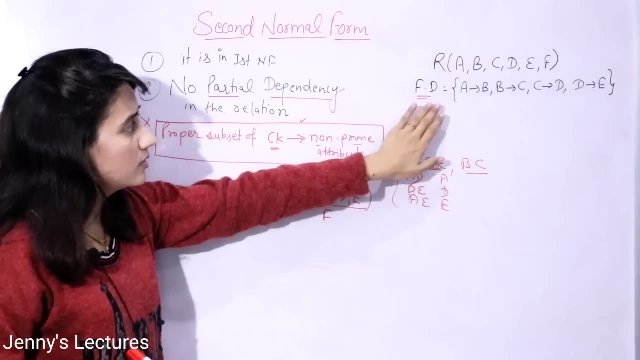 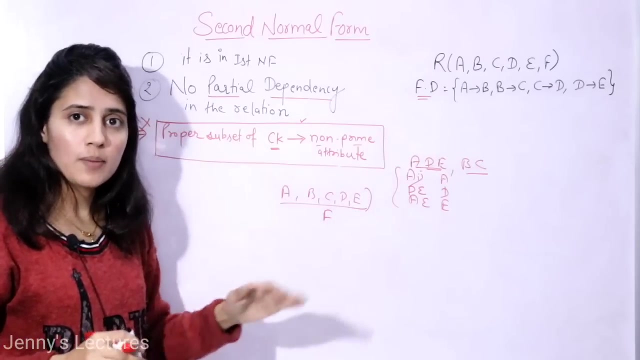 attribute right. so i hope you got now what is known prime attribute. so now let us discuss it with this example. let us find out this relation is in second normal form or not, right, and after that we will discuss it with help of two or three examples, with all the type of examples. i'll take all the type of examples and after that we will. 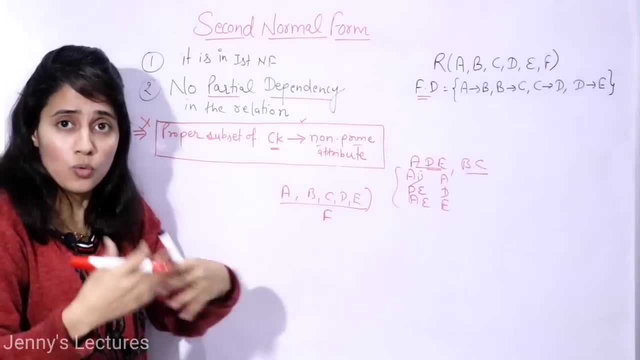 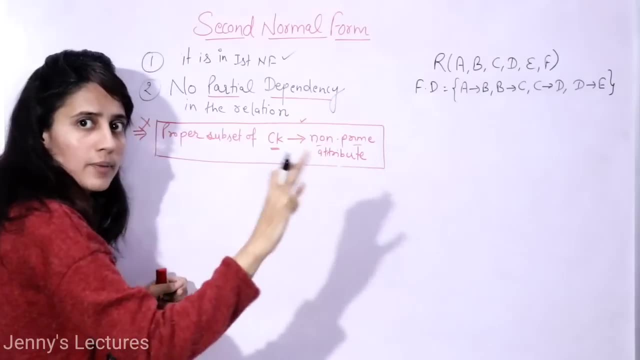 see if this is not in second normal form, then how to convert it into second normal form right. so now this is in first normal form, right. by default, the relational schema is given and this condition is satisfied. now you have to find out. this condition means there should be no partial 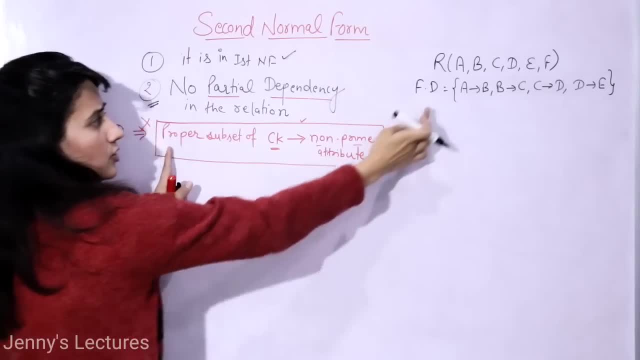 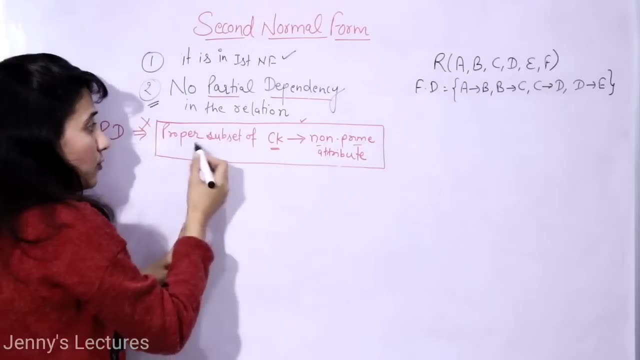 dependency. so now you have to find out this type of functional dependency here. if this type of functional dependency present here, then you can say this is not in second normal form right. but for this you have to find out what is candidate key to find out the proper subset of candidate. 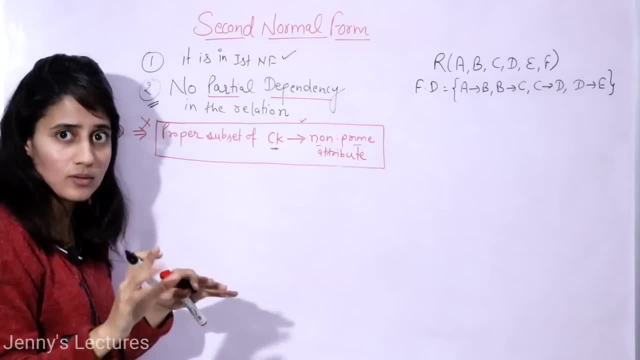 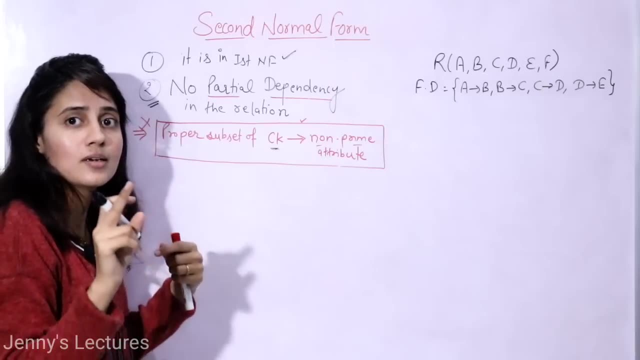 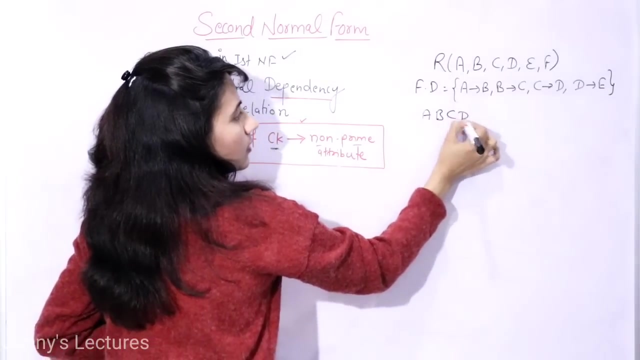 keys. you have to find out all the candidate keys from a relation right. without finding candidate keys you cannot do anything. so that is very important now how to find out candidate keys. we have already discussed candidate key is what? the minimal super key. so now now here how to find out by taking the attribute closer, so that also I have discussed what is. 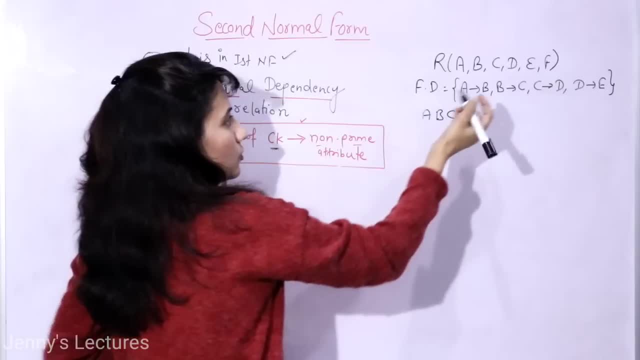 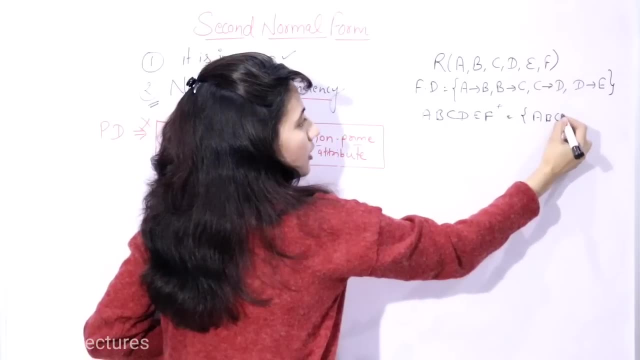 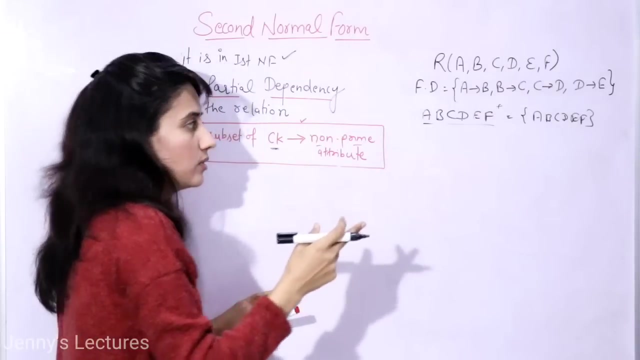 attribute closer and how to find out the attribute closer of an attribute right. so I will take first of all all the attributes, find out the closer. definitely it will find out all the attributes. so this is what definitely a super key right because of reflexivity property. now try to 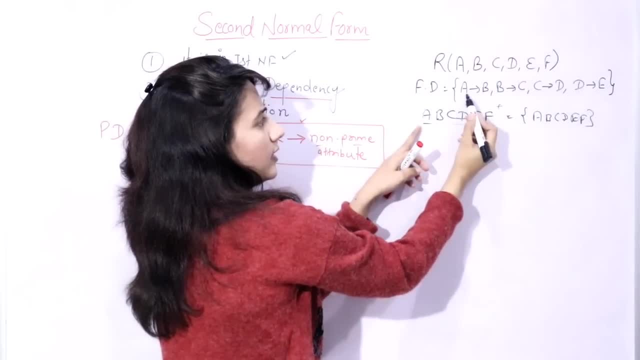 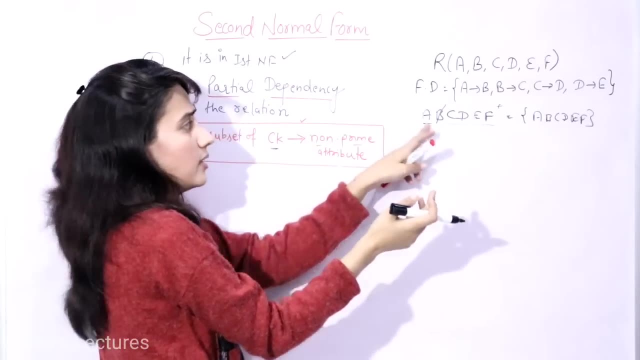 discard attributes from here. so now a can determine b, so we have a, so I can discard b from here. because if you have a, then a can determine itself and a can determine b also, so you can discard b. a can determine b, b can determine c, so by transitivity property a can. 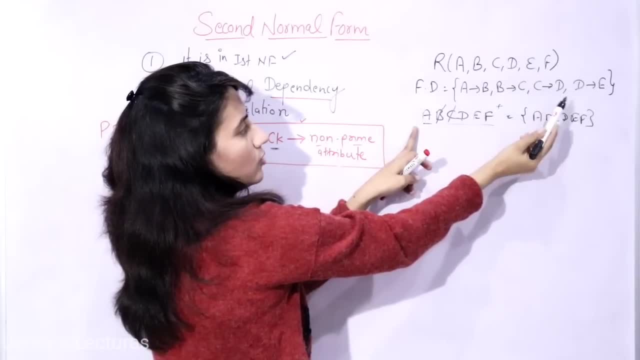 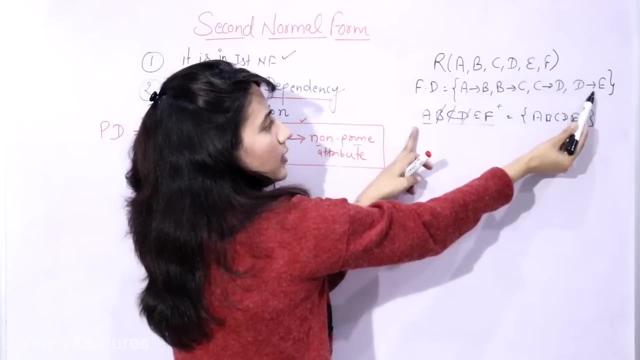 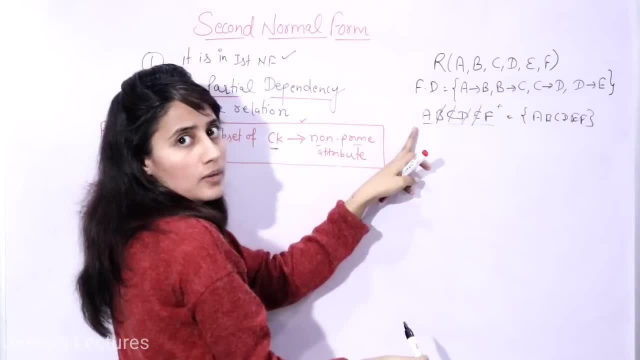 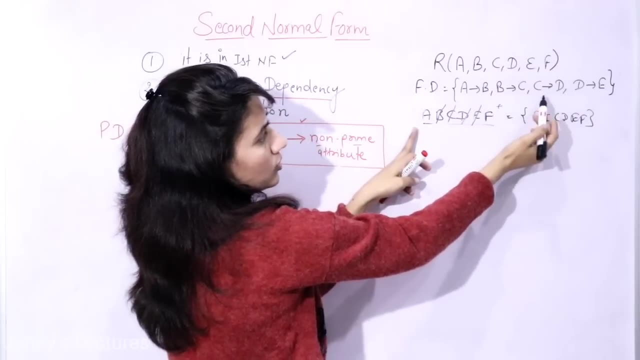 e. so by default a can determine e. so by default a can determine e. so by default a can determine e. means by transitivity property, so you can discard e. can you discard f? no, we don't have such type of dependency that using that we can discard f because nothing is going to find out. 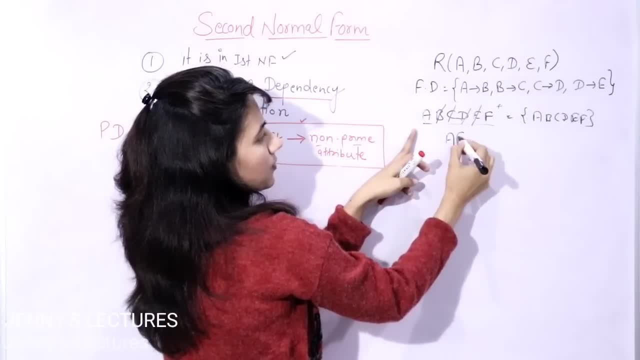 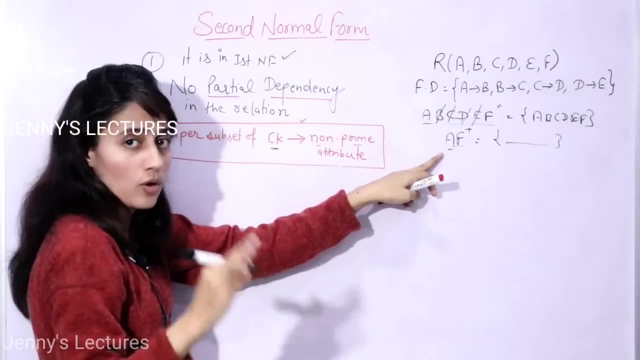 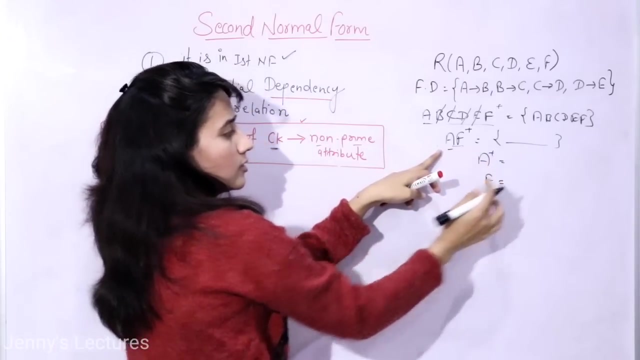 nothing is determining here, f. so now a and f. you can take the closer and you will find all the attributes. so this would be the super key, right? so how to find out that that is candidate key or not? proper subset is a and f. proper subset is: if proper subset is also super key, then that would not be a candidate key. 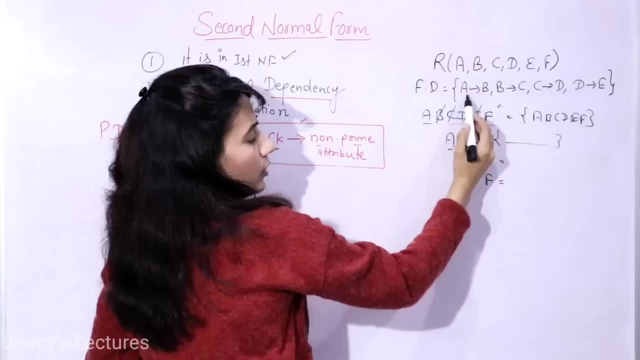 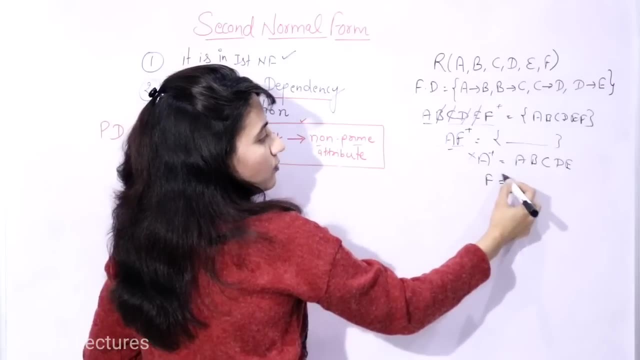 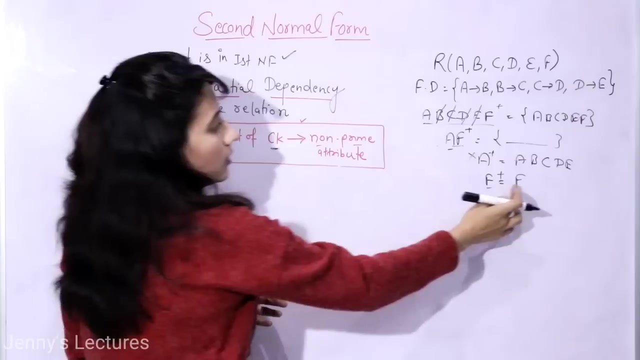 you can find out closer of a, closer of a will find out a right itself, then b, then c, then d, then e, not f. so this is not super key. f, proper f, closer would be what only f, f can determine itself. this is trivial, functional dependency, nothing else. so this is also not super key. so here you can say: 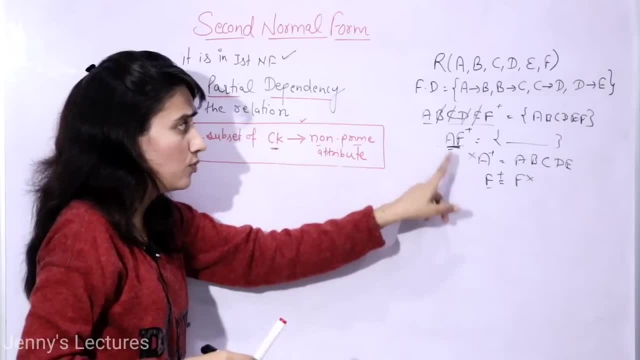 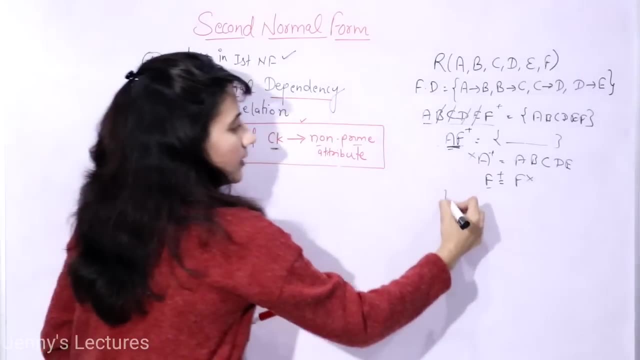 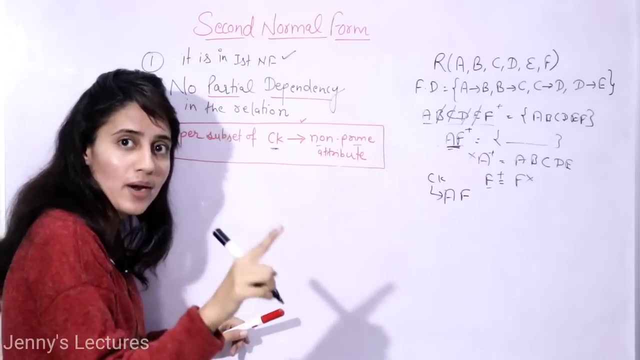 a f is candidate key because it is not a candidate key. it is not a candidate key. it is not a candidate key. it is no proper subset of super key. this super key is super key, right. so here, a f is what candidate key? we have got one candidate key, that is a f. so now we have got, as well as the prime. 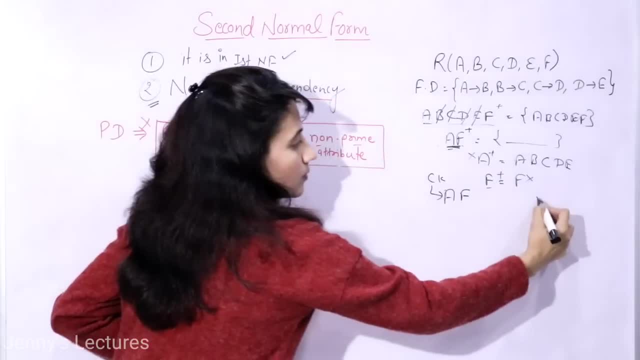 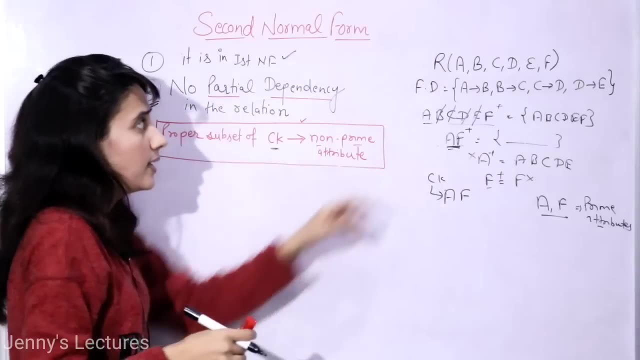 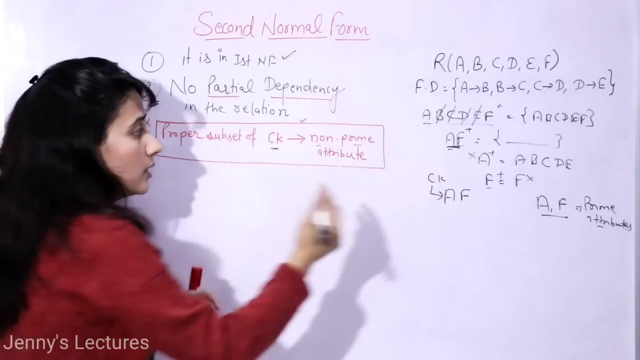 attributes. right means a and f. a comma f are prime attributes. now you have to find out- still there are another, more so more candidate keys exist in the relation or not, because we have got only one candidate key. now how to find out that thing if the prime attributes are present? 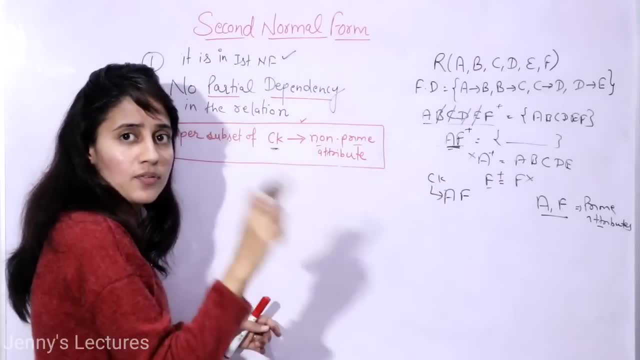 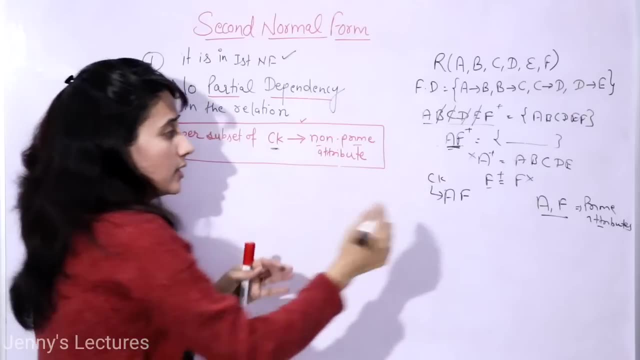 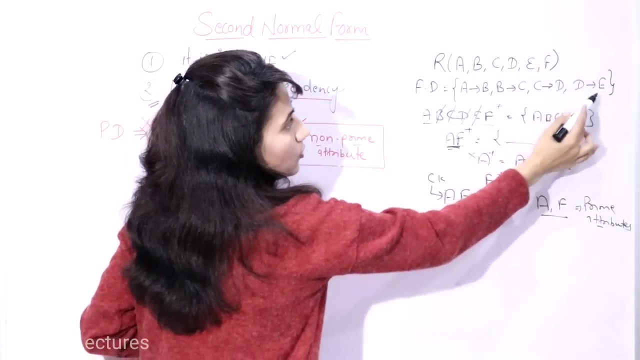 on the right hand side of any functional dependency, then definitely there would be more candidate keys present. if not, then there would be no more candidate key. so find out: is a present on the right hand side of any functional dependency? no, f, no. so in this relation, only one. 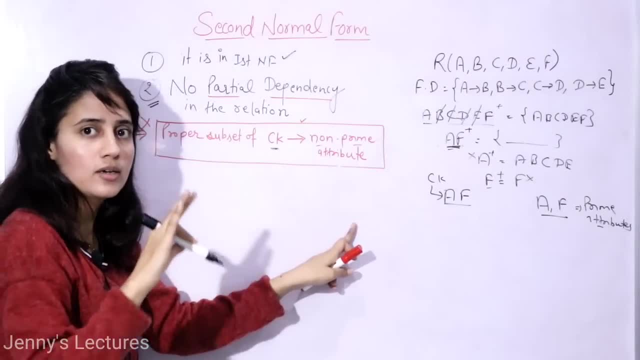 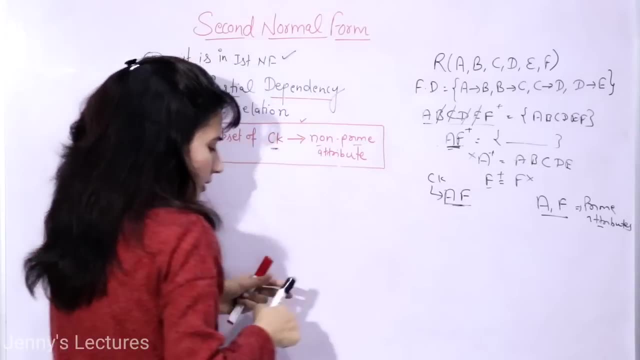 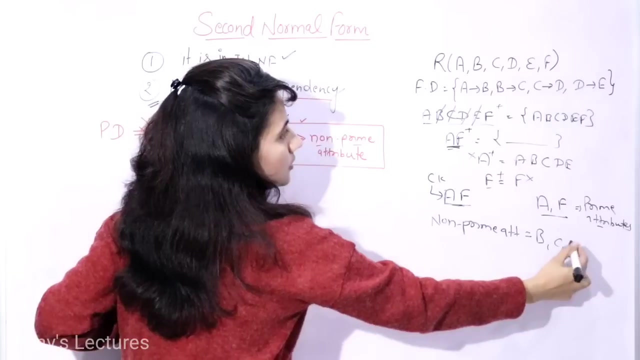 candidate key is there. that is a, f, no more candidate key. you will find right, that is the short trick. fine, now, if a, f is candidate key, then here known prime attributes are: a, f are prime attributes, so remaining means b, c, d, e. these are known prime attributes. 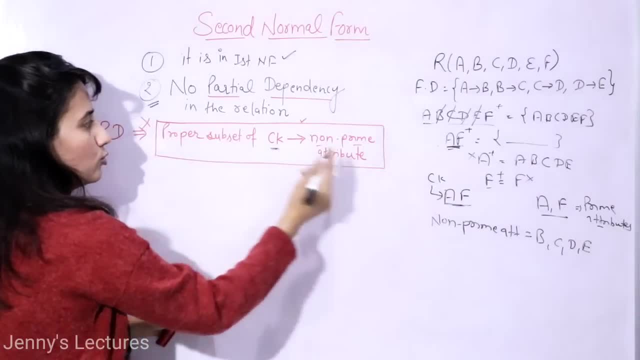 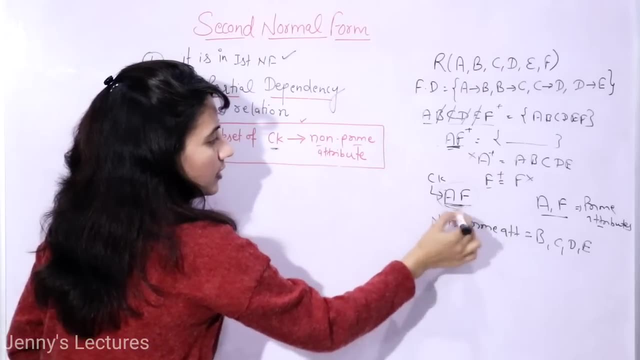 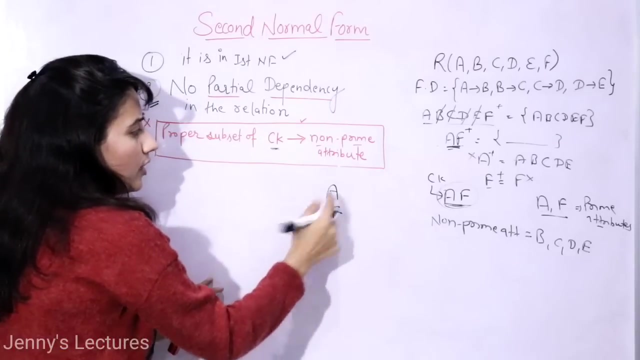 now we have known prime attributes also and candidate key also. now you can check out this type of dependency exist here or not. see proper subset of candidate key. proper subset of this candidate key is what? because i have only one candidate key, a and f. right. is a or f determining any known prime attribute? see here, f is not determining. 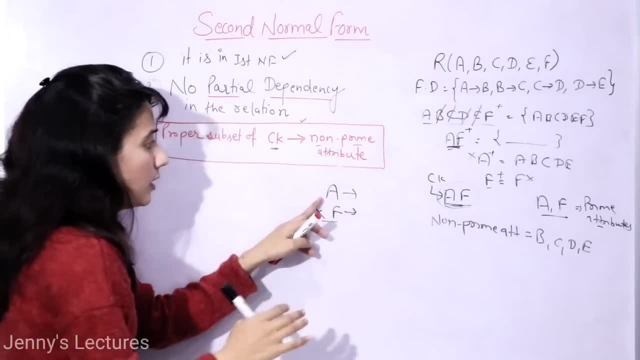 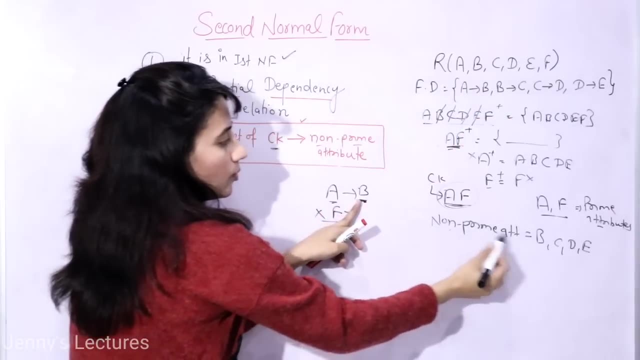 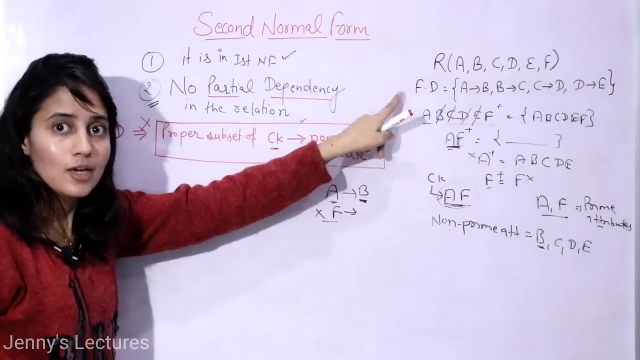 anything. so it cannot be there. it cannot be a case now. is a determining here c, a is determining b right and b is what known prime attribute means. you got this type of functional dependency here, right. so this is what a determine b and a determine a right. so this is what a determine. 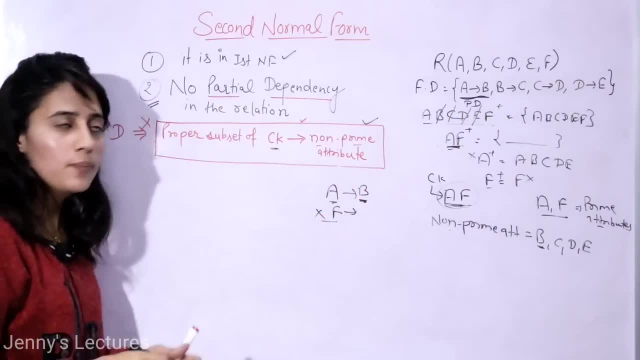 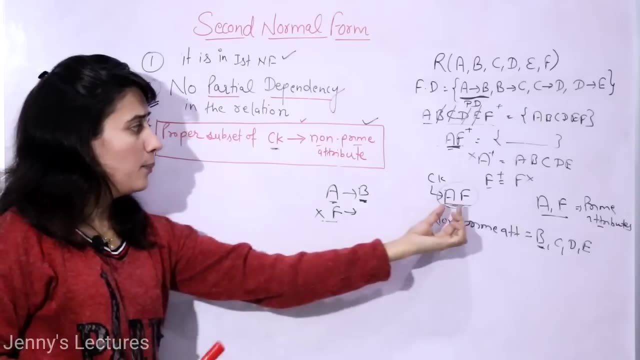 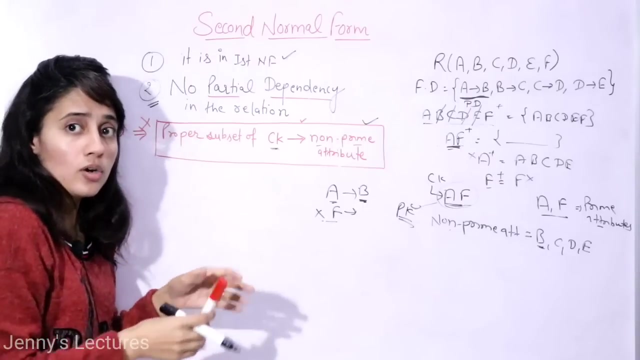 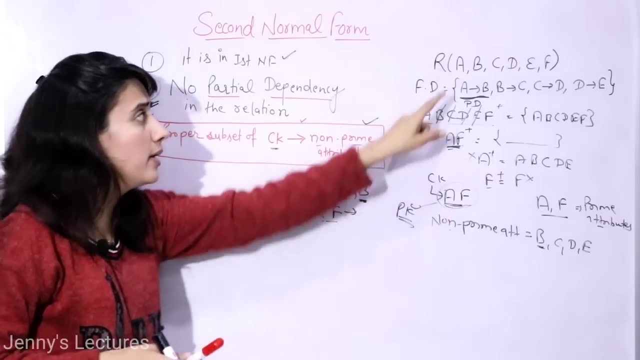 b. this is what partial dependency. so here partial dependency exist. so this relation is not in second normal form, or in another word you can say: see complete a f is candidate key and definitely it is also primary key right. and only a part of this primary key, only a part of this primary key or candidate key, is determining a known prime attribute. 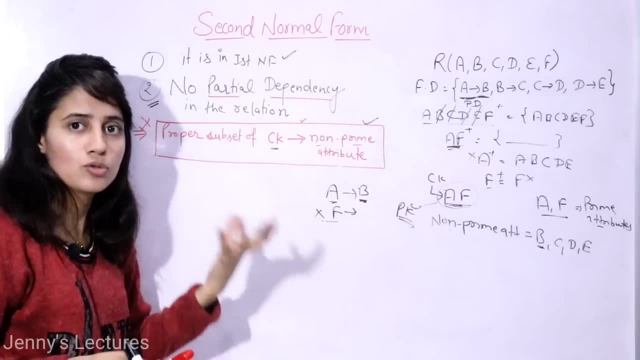 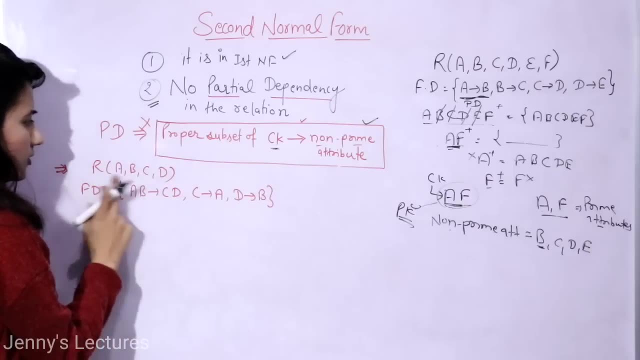 only a part, not the complete candidate key. so that could not be possible, right. so now let us discuss it with one more example. so let us take this example now. this is the relation having four attributes and these are the functional dependencies given here. so this relation is definitely by default in first, normal form. 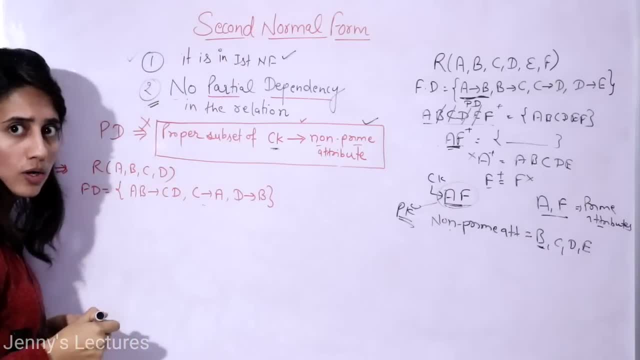 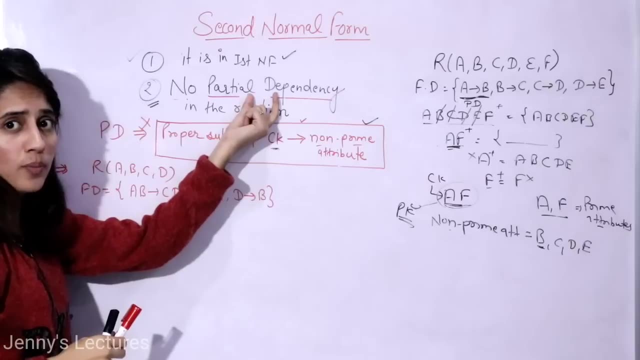 right now you have to check the partial dependency present here or not. how to find out partial dependency. see this thing you have to take care. if you know how to find out partial dependency, what is partial dependency, then you can easily find out that partial dependency is not a part of 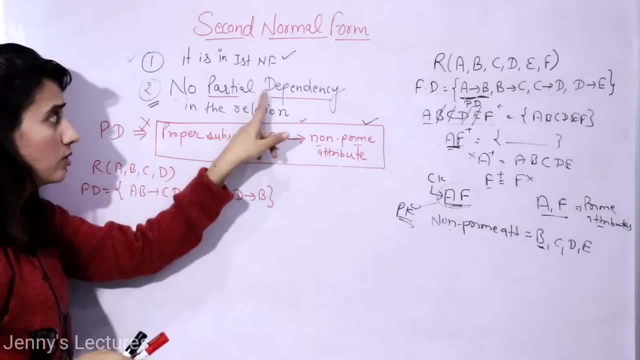 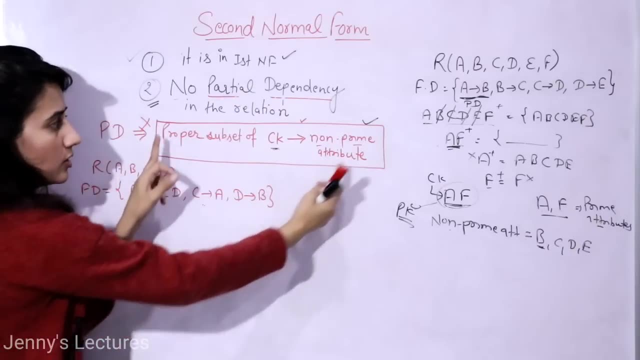 a particular relation is in second normal form or not. this is the important concept here, right? so partial dependency means you have to find out this kind of dependency in the given list. for this kind of dependency, you have to find out candidate keys, all the candidate keys, and definitely then you can. 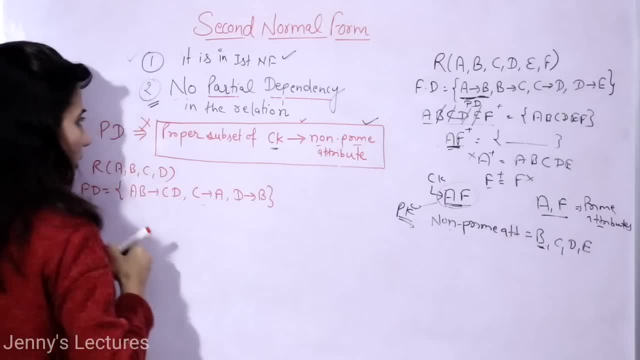 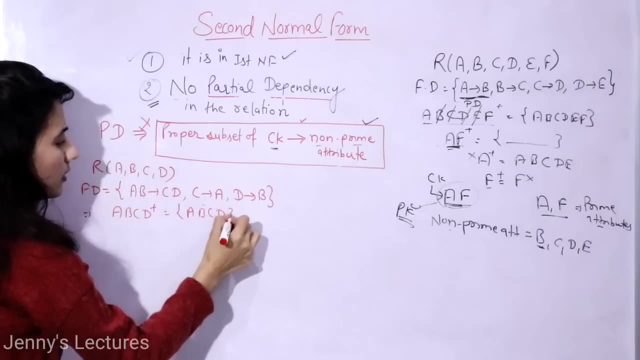 find out the non-prime attributes right. so now, first of all, find out the candidate keys. how to find out? take all the attributes, take the closer and all the attributes definitely would be super key right now. try to distinguish between the candidate keys and the non-prime key right now. 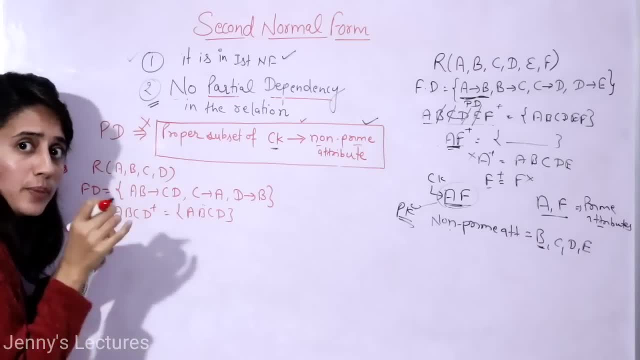 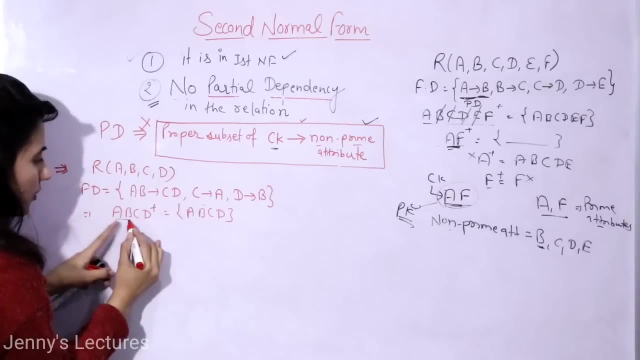 check the dependencies: a b, both can determine c? d. do you have a b? yes, i have a b, so i can determine both c and d. so a b closer would also find out a b itself because of reflexivity. and a b can determine c? d. do you have a b? yes, so i can determine c d. so this closer of this a b. 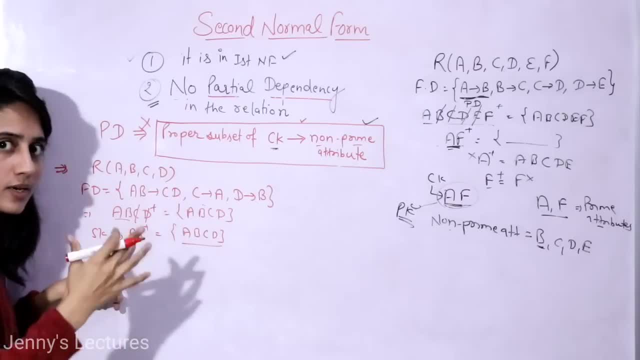 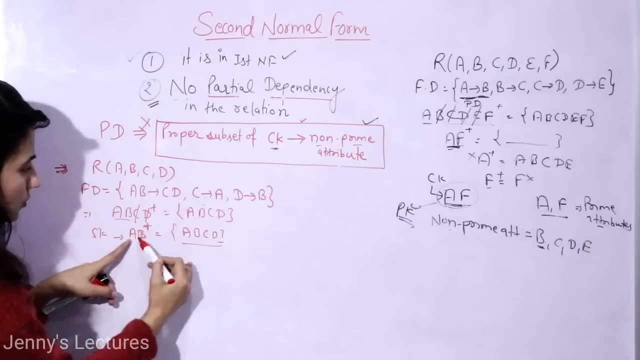 is containing all the attributes. so a, b is what super key? a, b is still a super key right now. can you discard any more attribute from a, b? c can determine a you have. do you have c? no, d can determine b, but we don't have d. so we cannot discard any more attribute right. so now check. 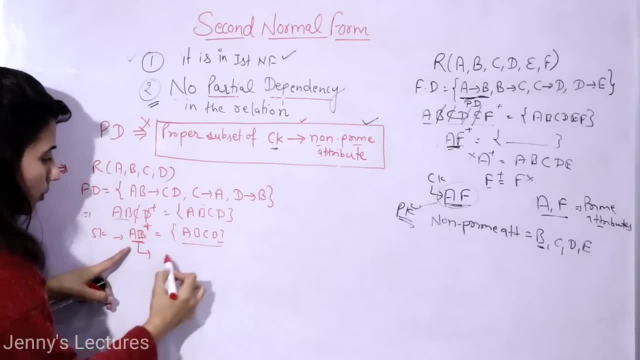 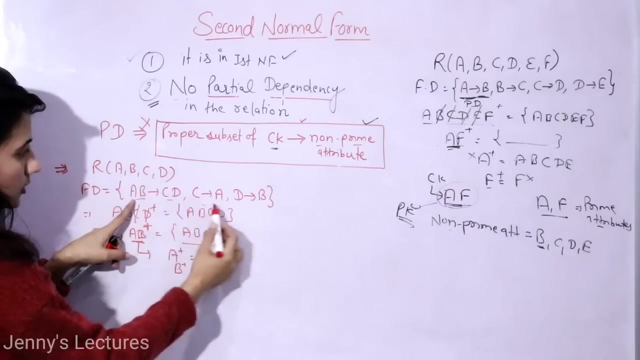 out as a, b's candidate key or not. find out the proper subset, that is, a and b. find out closer of a. find out a and b individual can be a super key or not. closer of a single: a can determine a, but we don't have a- b, so we cannot determine c, d. 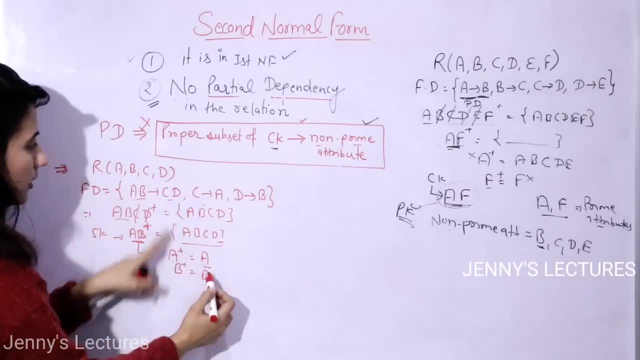 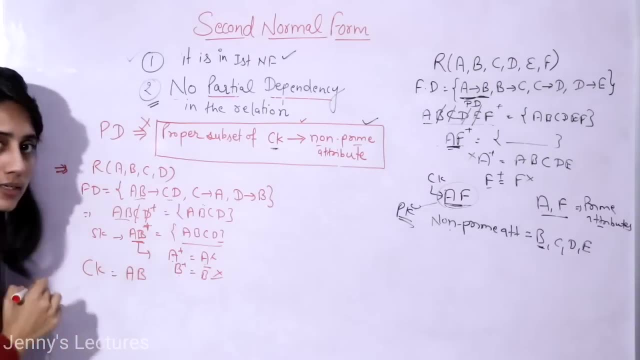 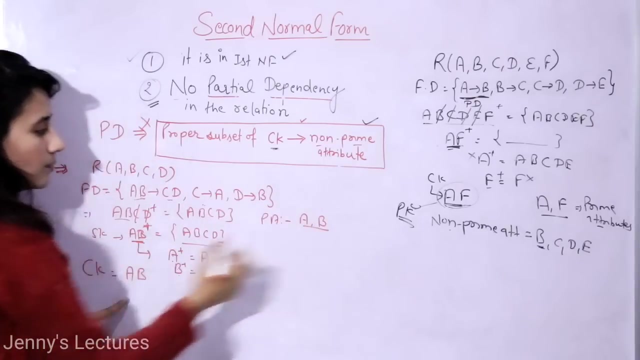 only a can determine only itself. b can determine b, only b. so this is not super key. this is not super key, so it means candidate key: a, b is what candidate key? we have got one candidate key. it means prime attributes are a and b. right now check more candidate keys are present or not. 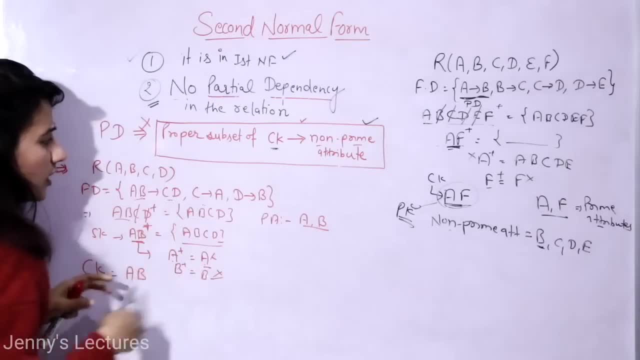 how to check. if prime attributes are present on the right hand side of any functional dependency, then definitely more candidate keys would be there. see a is present on the right hand side of this functional dependency. right means you will get more candidate keys here right now. how to do that thing: see existing candidate key is this one. so at the place of a, you can replace a. 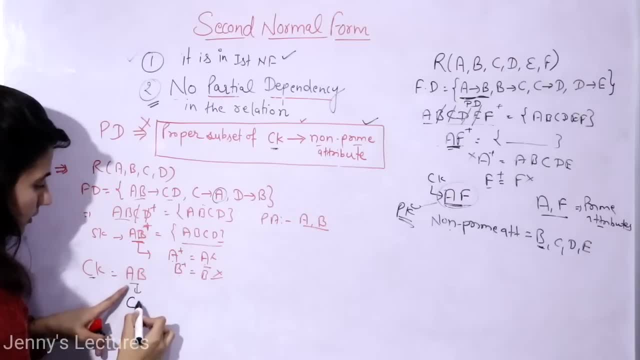 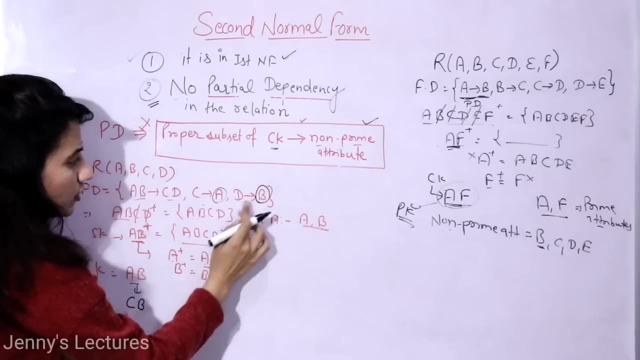 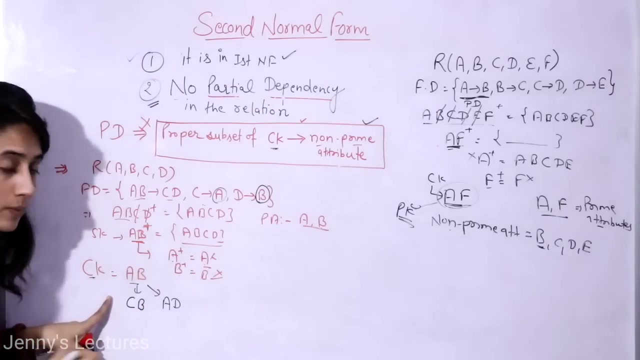 with c after replacing, you will get c b right. and second option is: see: b is also prime attribute and b is present on the right hand side of d. so second option is: at the place of b you can write down d. now you will get. what does that mean? trazer it to another cell? and we have not seen that. 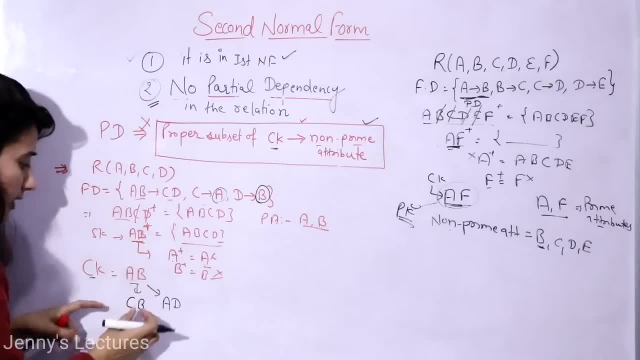 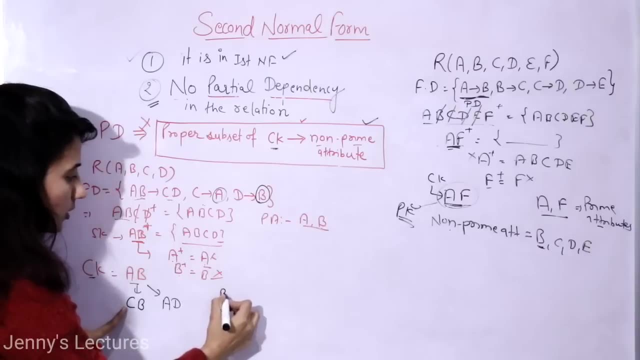 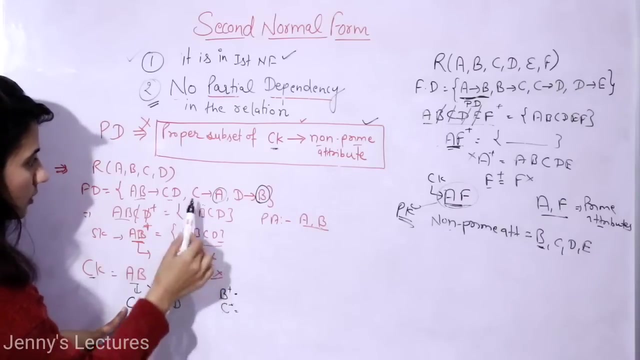 this point here you can write down d be present in any un correspondent state. another slide and on the second option you will get size and size right. so the next problem I have with this project solution: I think it's very complicated, right this and this would be definitely candidate keys. still you need to find out. but yeah, I can say that. 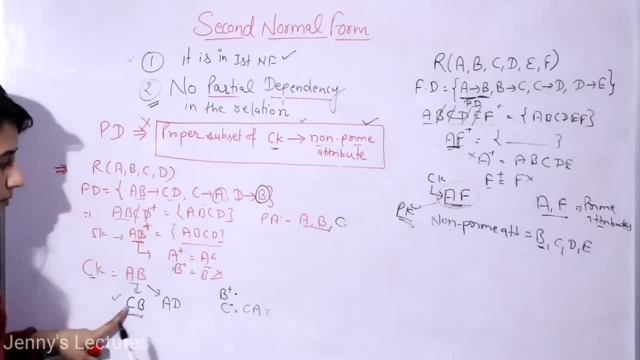 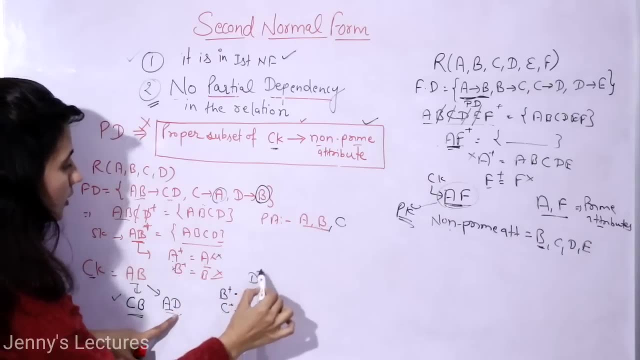 So now we go to one more prime attribute, that is C. Now check out A: D is candidate key or not. A closer, not candidate key, D closer, D closer can find out D and B, nothing else. So this is: 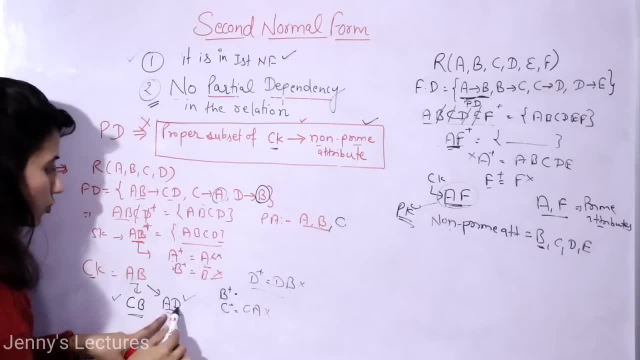 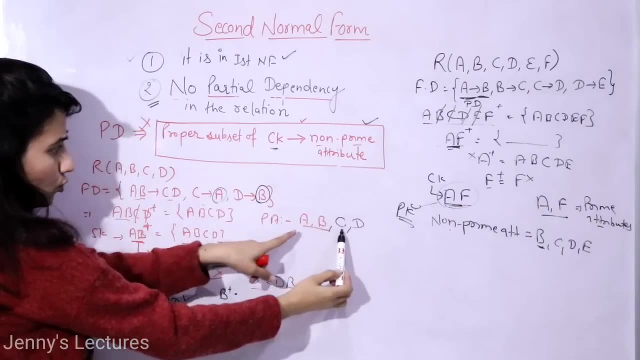 also not super key. So this is also candidate key here. fine, So A and D. So D is also prime attribute right Now you can check. we have got two more prime attributes Now check these are: 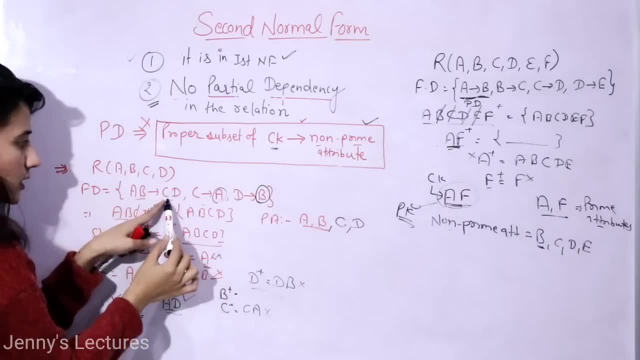 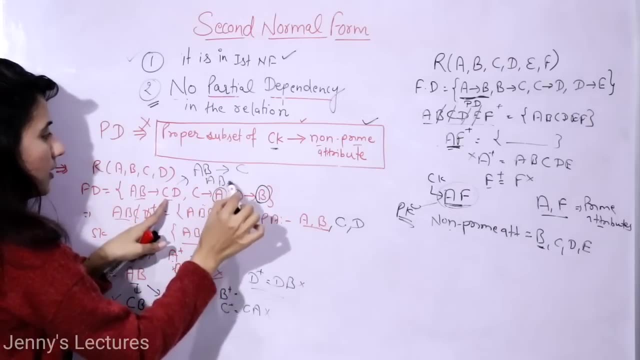 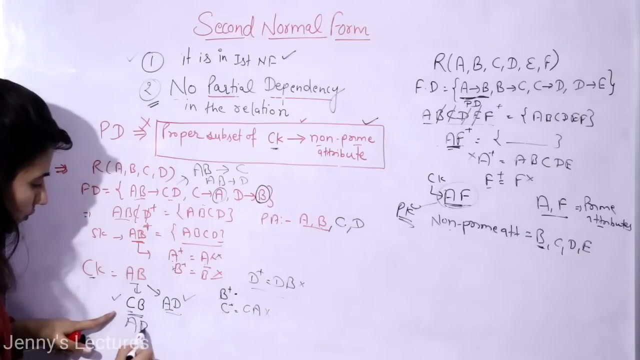 available on the right hand side of any functional dependencies or not? Yes, available, See this. you can write down something like this: By splitting property, A B can determine C and A B can determine D. So at the place of C you can replace it with A B Here A B. So obviously we will. 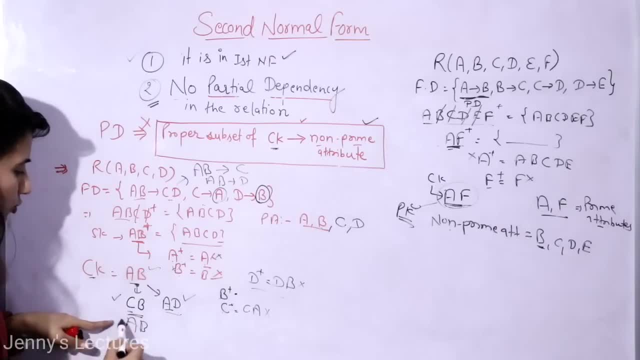 not write A B, B, A B, but we have got on the candidate key A B, So no need to replace. And at D also A B, at D also A B. So we have already got A B, So no need to replace. 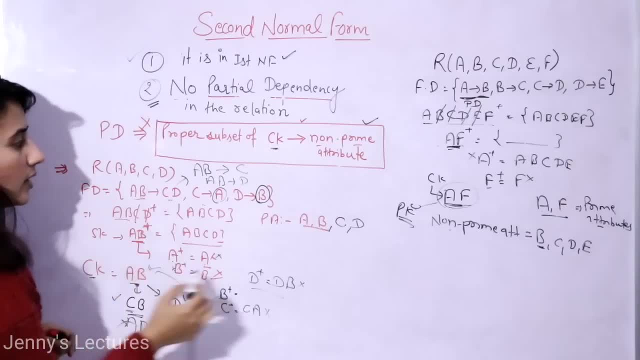 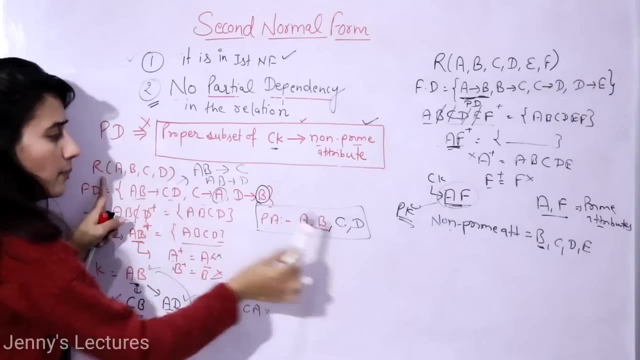 So now these are the candidate key. three candidate keys in this relation and prime attributes are A, B, C, D. Now here all the attributes of the relations are prime attributes. So definitely that relation would be in second normal form. 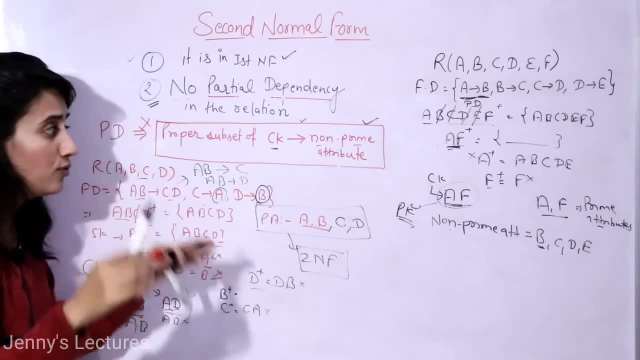 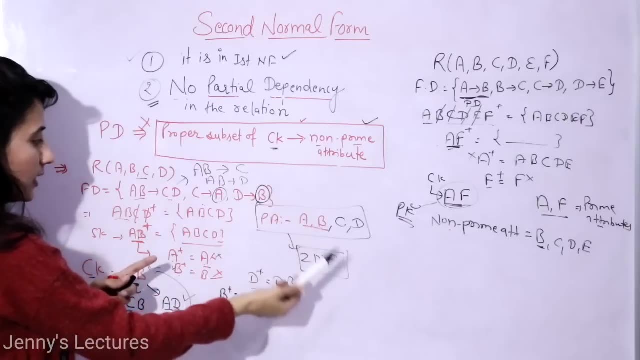 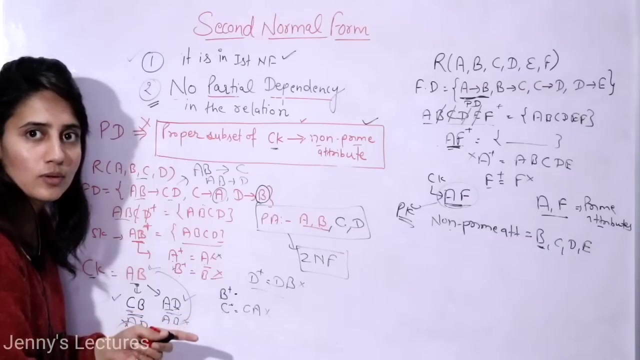 Why so? Because there is no known prime attribute. If no known prime attribute, then you will never get this type of situation, Because proper subset of candidate key is determining known prime attribute. This is partial dependency, but we don't have any known prime attribute, So you will never get this kind of dependency here. Right, See at the right. 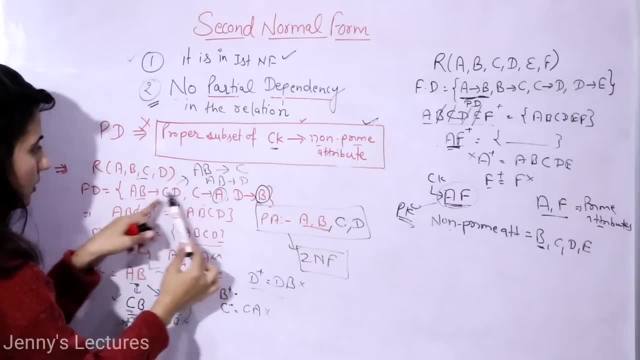 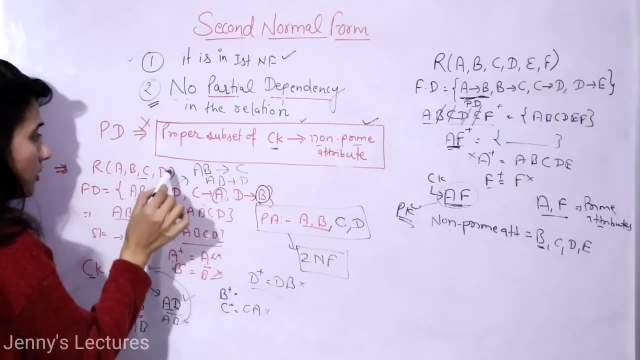 hand side known prime attribute should be there. You can check. Right hand side is C D, but C, D is prime attribute. A, A is also prime attribute. B, B is also prime attribute. Fine, So if all, 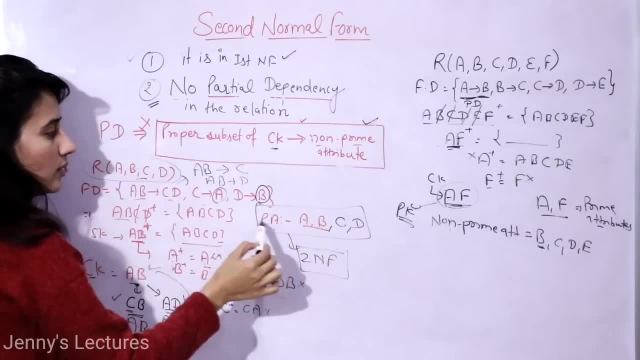 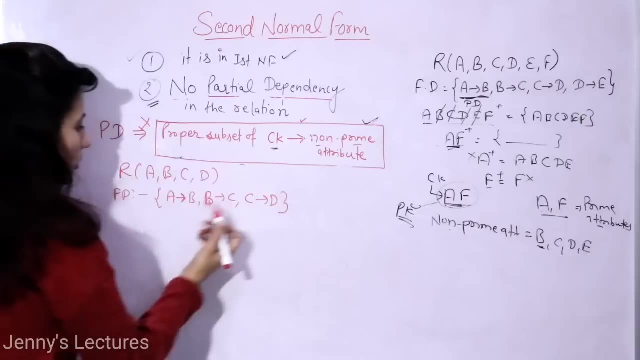 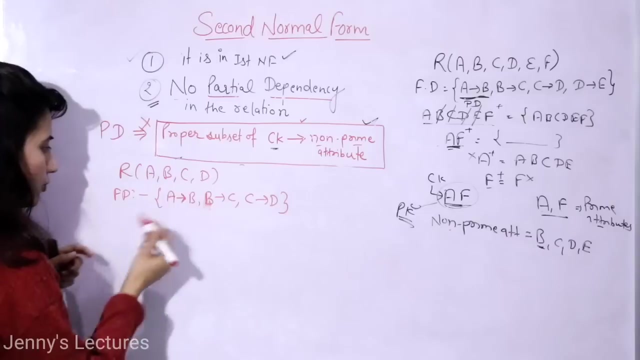 the attribute of a relation are prime attributes, then that relation is definitely in second, normal form. Fine, Let us start. Let us take third example. So third is this type of question. Four attributes are there in our relation. These are the functional dependency. Find out the candidate key, first of all. How to 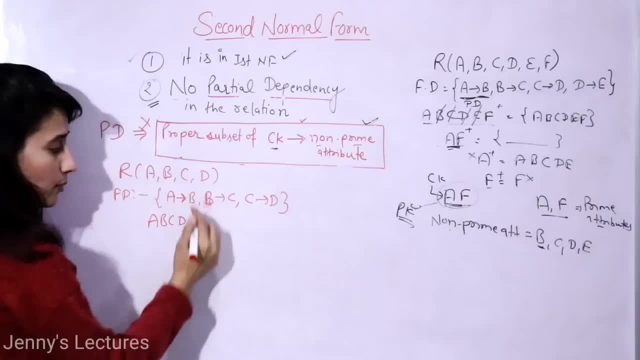 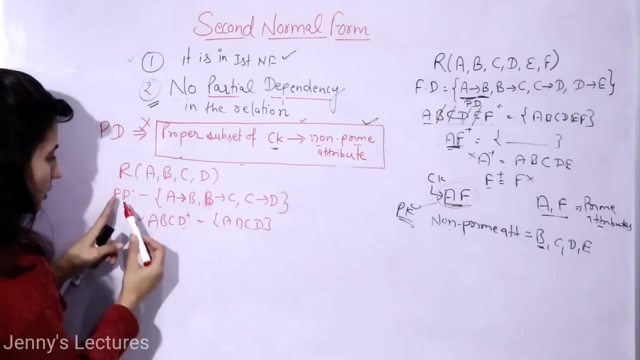 find out. Simple rule: Take all the attributes. Obviously, the closer would be A, B, C, D. Find out all the attributes. So this would be super key Right Now. try to discard attributes. How to discard. Check the functional dependency: A is determining B, So do you have A? Yes, 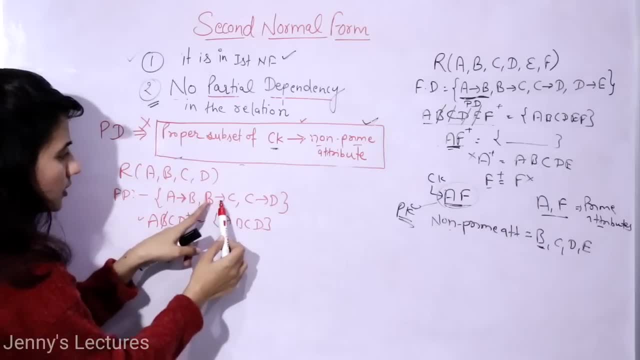 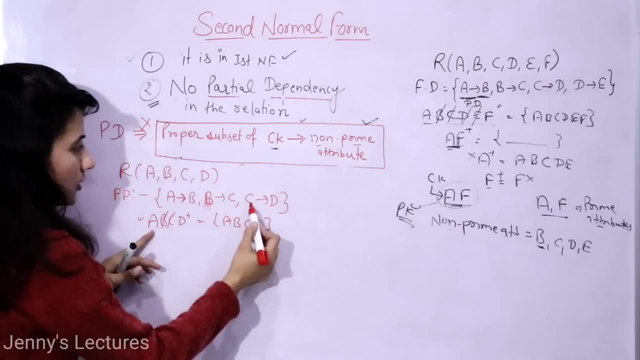 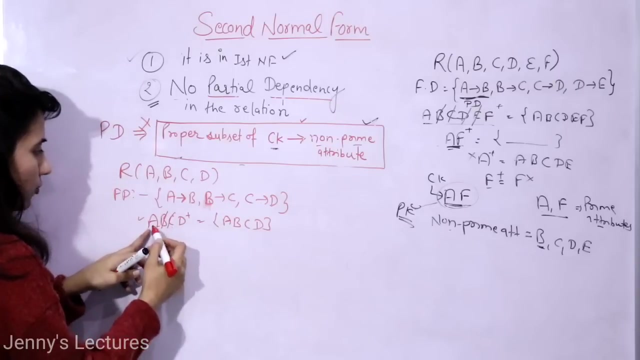 I can discard B. A is determining B, B is determining C. So by transitivity property A will determine C, So I can discard C because I have A. Now. third is what C is determining D? Means A can determine C and C can determine D by transitivity property. So means here you have A. 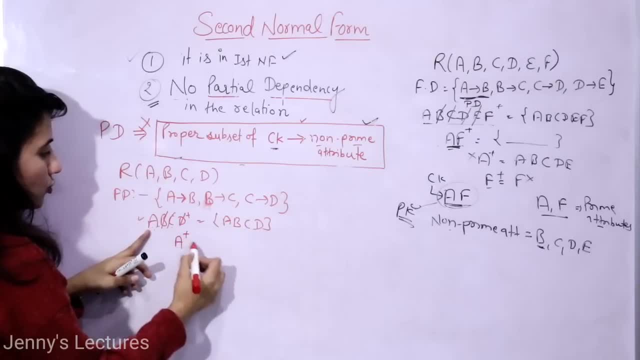 So you can discard D. So now we are left with only A, So find out A closer. Is it super key or not? A will determine itself. So we have A. A will determine B. Do you have A? Yes, So it will. 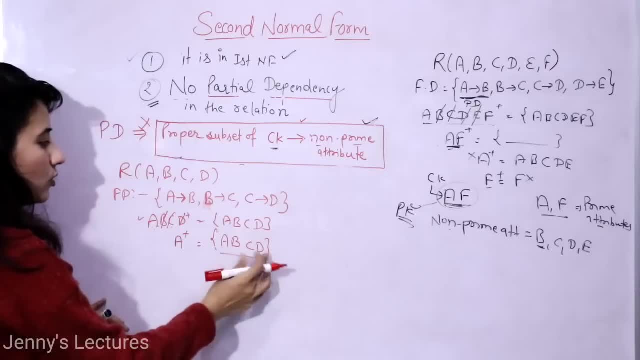 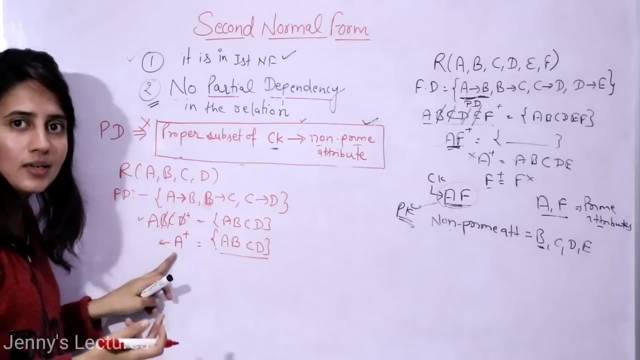 determine B, B will determine C, C will determine D. So I am getting all the attributes of a relation. So A is what Super key Right Now? is A candidate key or not? Definitely yes. Why so? Because proper subset of this. 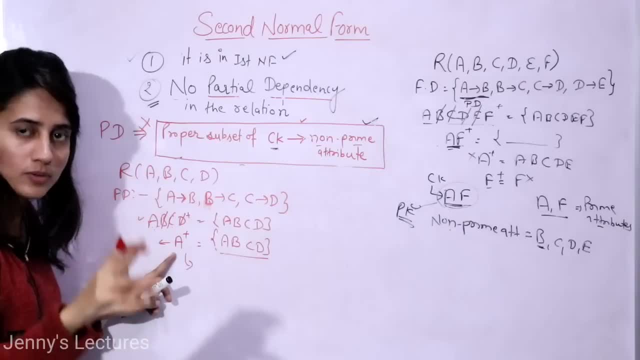 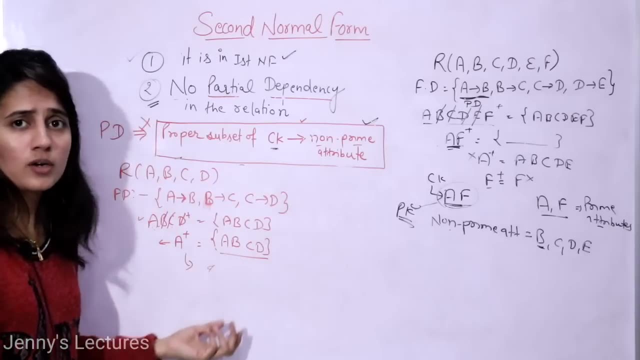 A is what Phi? only Right How to find out proper subset. That also I have discussed in the previous video. You can check out that video in the side button Right. That is phi and phi set of attribute cannot determine any attribute of a relation, So definitely. 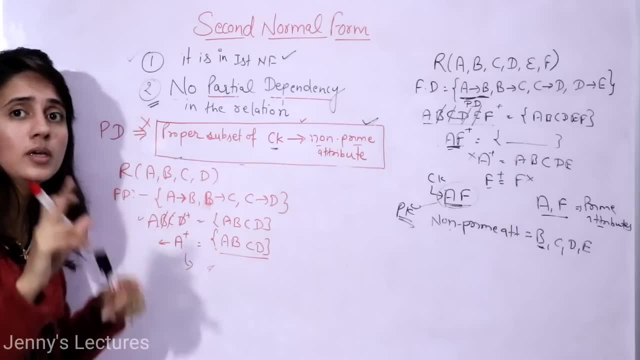 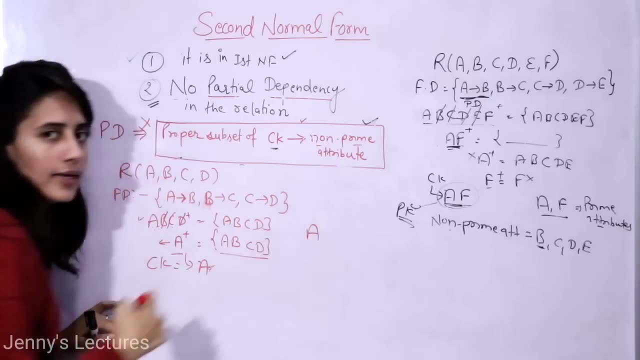 if one attribute is there in a super key, then definitely that would be candidate key. So here A is what Candidate key? So prime attribute. we got A. Now check: Prime attribute is available on the right hand side of any. 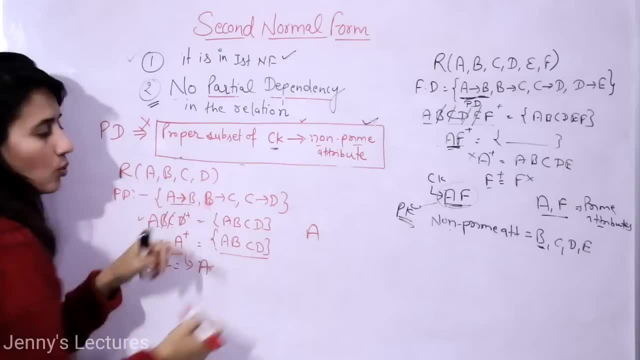 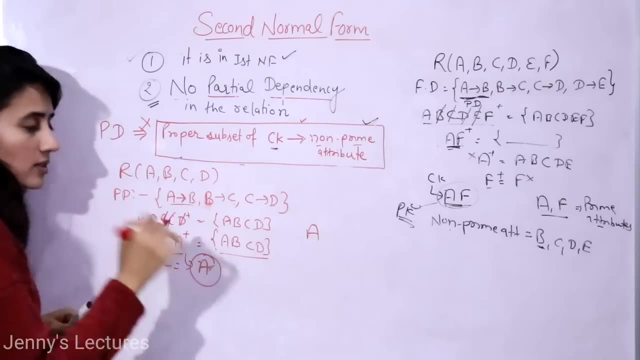 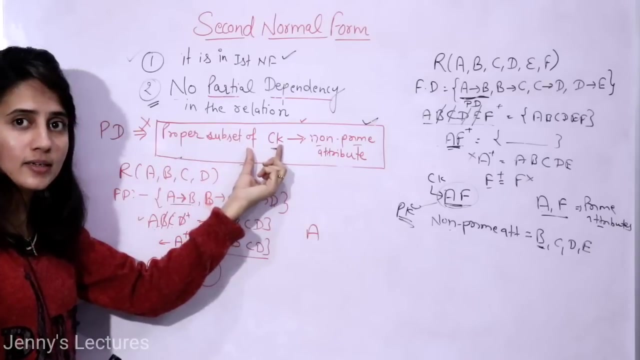 functional dependency. Here we have B, Here we have C, Here we have D. No, It means there would not be no more candidate keys. Here we have only one candidate key, that is A. Now see here candidate key is having only one attribute. So proper subset of candidate key. Can you get any? 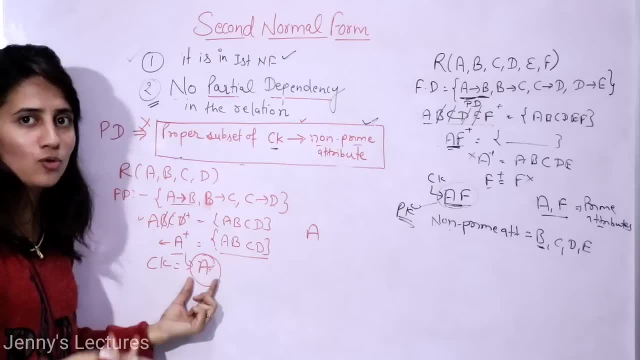 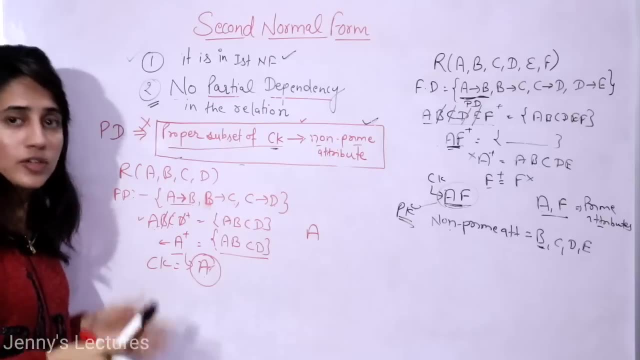 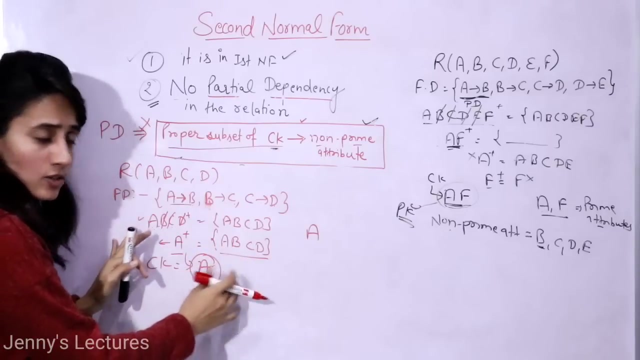 proper subset of this. Proper subset would be what Phi, only No attribute would be there. Right Now there is no proper subset of candidate key, So definitely we will never get this kind of dependency here. So there is no partial dependency. 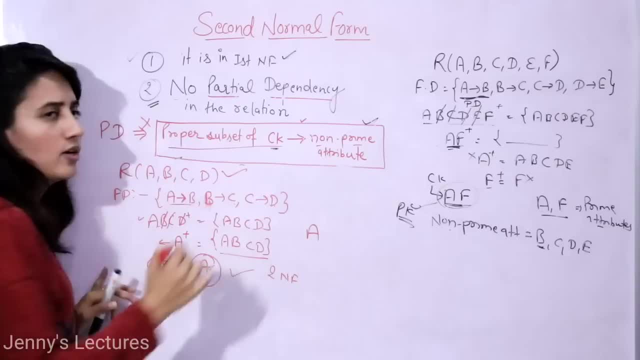 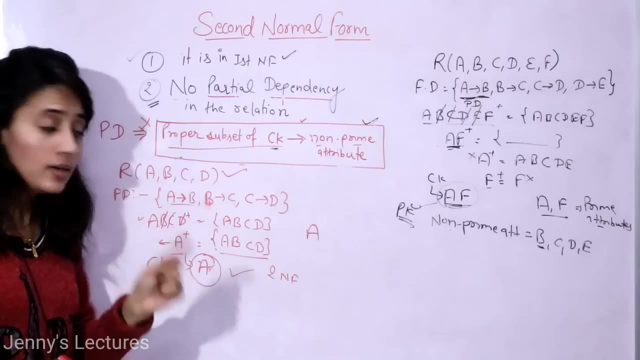 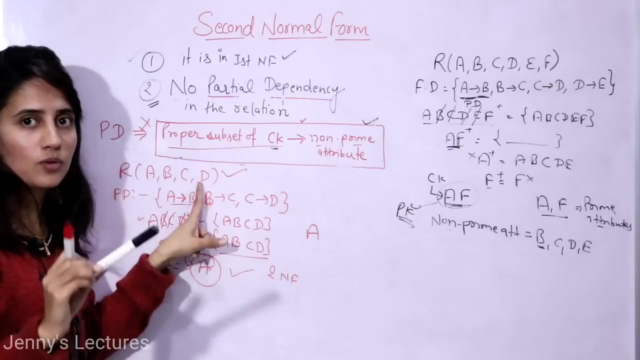 So this would be in second normal form. This relation would be in second normal form. So you can say something like this: If candidate key is having only single attribute, single attribute Right in second normal form, right, it's not like that. maybe. maybe in some case in some relation one. 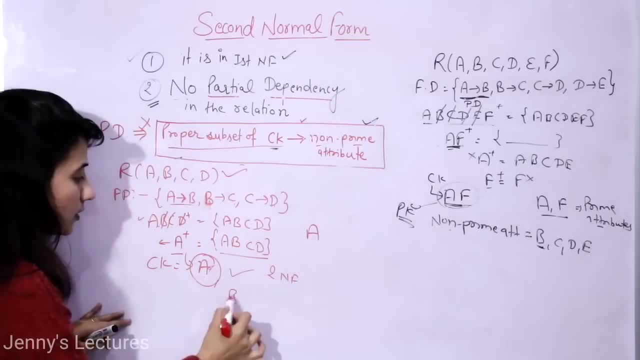 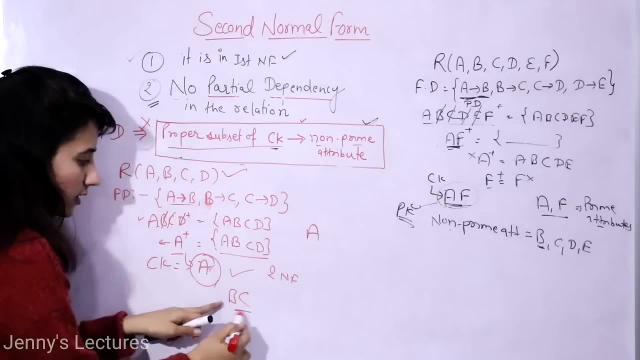 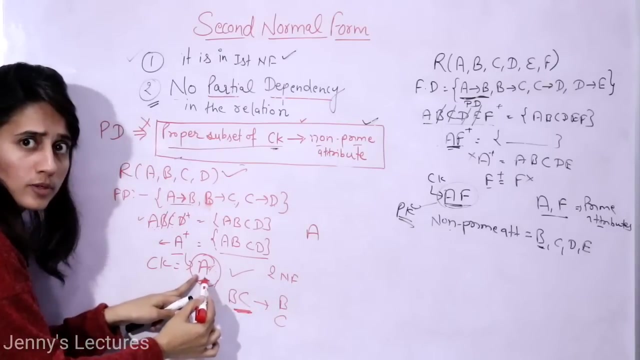 candidate key is having single attribute, another candidate key is having two attribute. in that case you cannot say that there would not be any partial dependency because one candidate key is having two attributes. so you can find out proper subset of this, you can. you cannot find out proper subset of this, but you can find out proper subset of this right. so it means 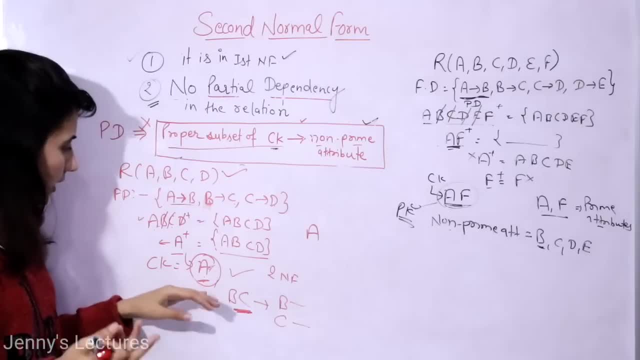 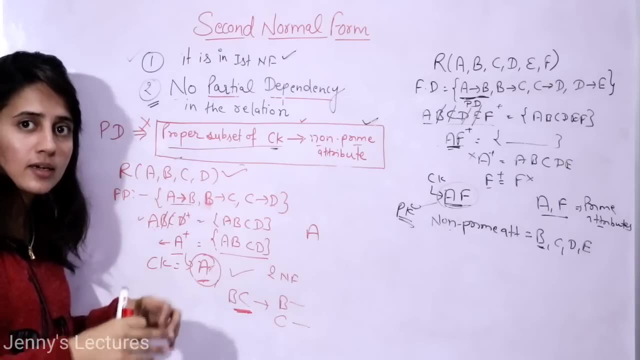 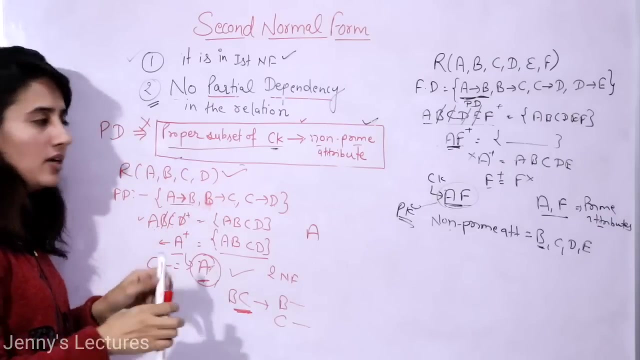 if all the candidate keys here- luckily i have only one candidate key- but if suppose all the candidate keys, two candidate keys are there, or three candidate keys are there and all the three candidate keys are having single, single attribute, then definitely there would be no partial dependency and definitely that relation would be in second, normal form. now i hope you got how to find out. 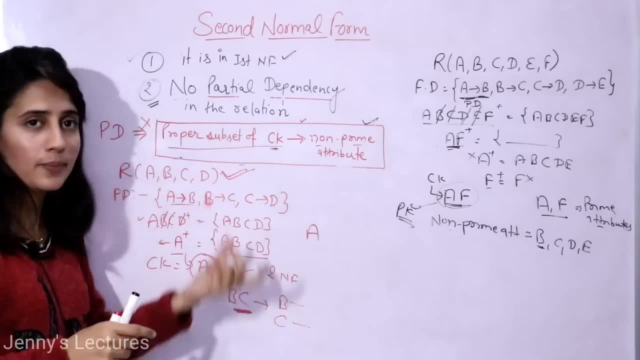 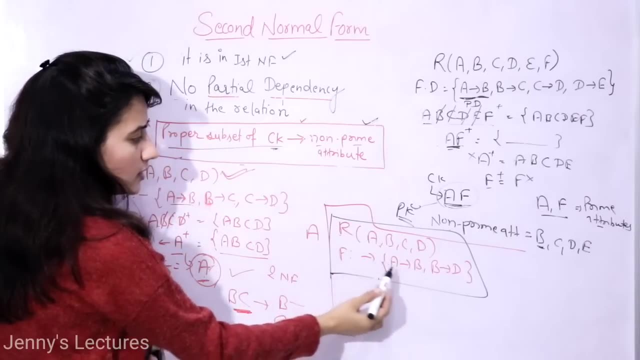 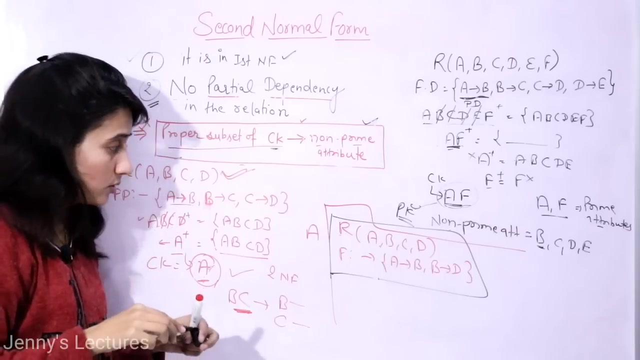 that particular relation is in second normal form or not right, and what is partial dependency? now see, one question for you. is you here this? this is the relation given and functional dependencies. are two functional dependencies only, a to b, b to d? i think this is very simple question, so you can tell me in the comment box that this.